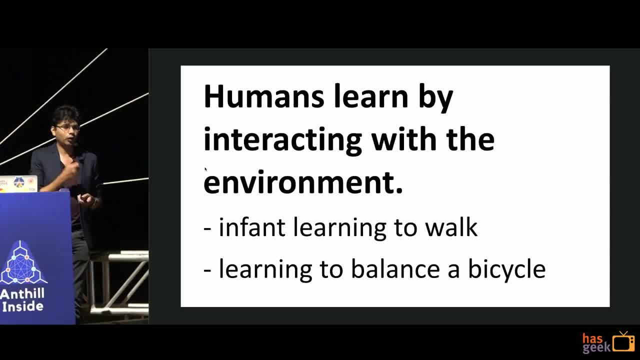 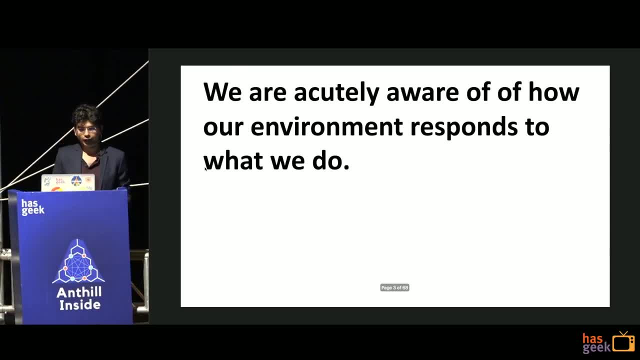 there's no explicit teacher as such saying: okay, this is one zero, one, zero, one zero in a conventional machine learning framework. yeah, and that's essentially going to be the motivation for reinforcement learning. and so at the couple of things here, right, as humans, we are acutely aware. 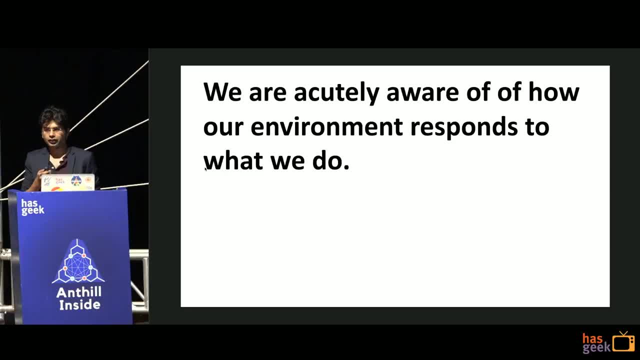 of how our environment responds to what we do. right, that's the key thing here. right, we are acting in an environment, we do something and we kind of get feedback right, so we know what the how the environment is responding to the actions we take. and second part is the most important part: 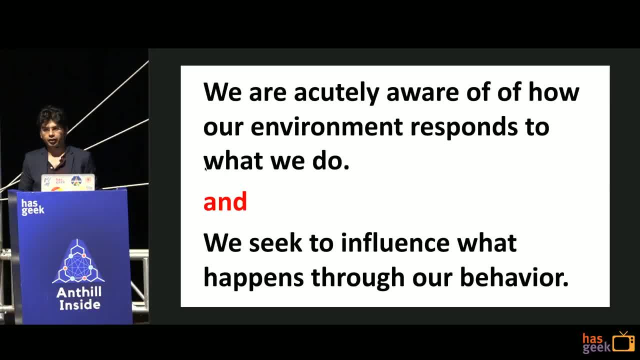 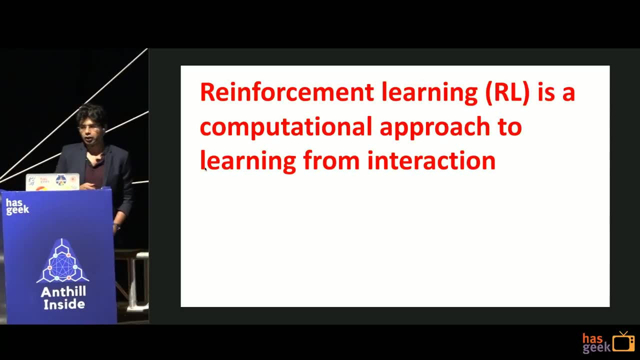 right, we seek to influence what happens through our behavior. right once you get the reward, i kind of now control how i should do my actions so that i can get my rewards better. yeah, so essentially a reinforcement. learning is just a computational approach to kind of formalize this. 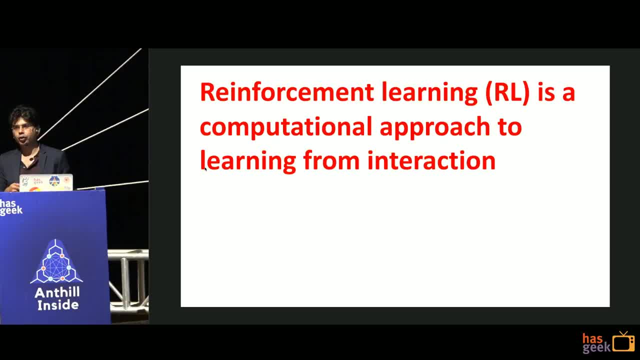 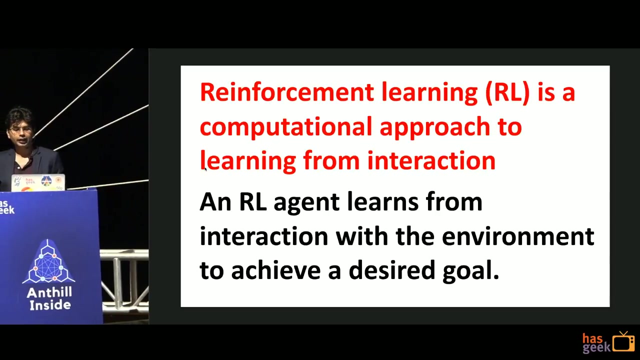 notion of learning practice with each creep & varieties. learning from interaction, yeah. so, in contrast with, you have this supervised learning where you're leaning from labels. that is unsupervised learning, no labels. so it's kind of the way to think is that this is a way of learning from interaction with the environment? yeah, 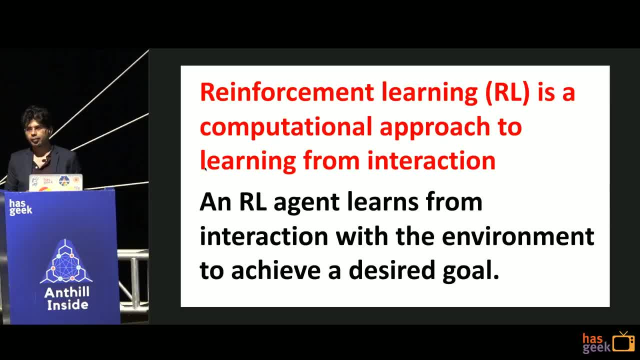 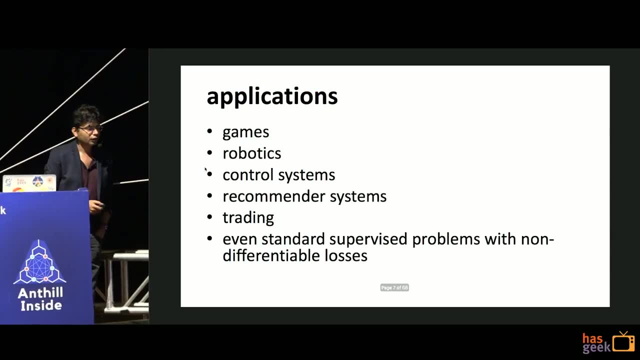 I think the rest of the slides are just going to be: how do I mathematically concretize this response statement? right, What is the mathematical formalism? for, just to make sure, how do you kind of model this statement? Learn from interaction with environment to achieve a desired goal? 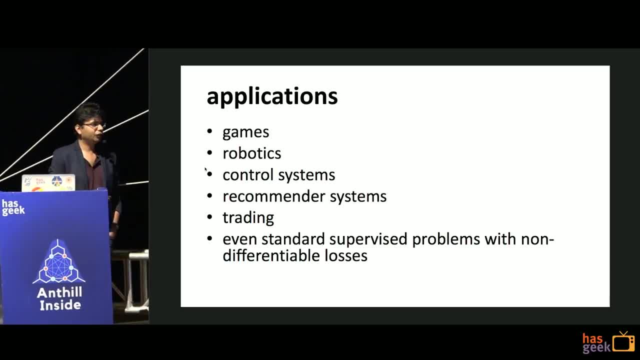 So there are kind of- I mean I won't go into lot of applications. There are quite a lot of applications like, for example, where this motivation is coming from, But I started with the way the humans learn as a motivation. But that's what not we are interested in. 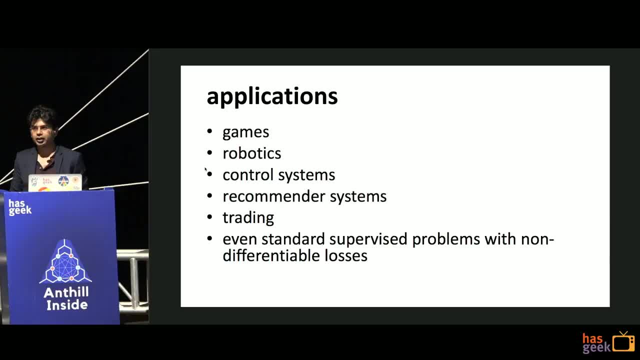 We are actually interested in lot of various problems. right For the classical example is learning to play games, control systems in robotics or even recommender systems. right can be cast in the deep reinforcement learning framework or even trading, or at a very high. 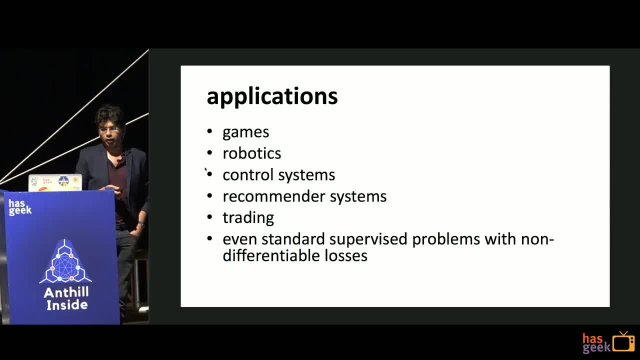 level, even some standard supervised learning problems kind of, if your problem with certain non-differentiable loss functions can also be cast as a reinforcement learning problem. yeah, So it is kind of a. it is a very new. I mean, it is not a new paradigm, but it is a very 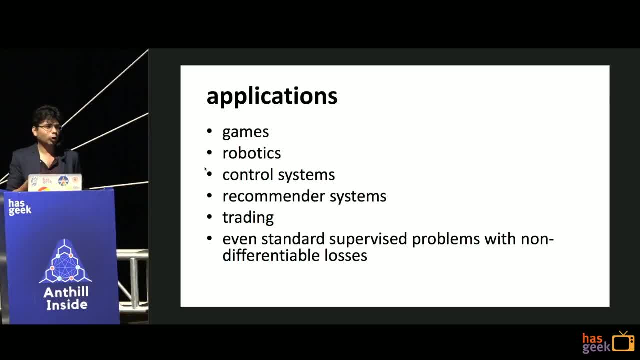 powerful paradigm if you somehow make it work. yeah, Because almost any problem you can think of, I mean you can cast it in a reinforcement learning problem, And that is what I want to get to you today. right, I will give you the basic formalism and you can think of your. 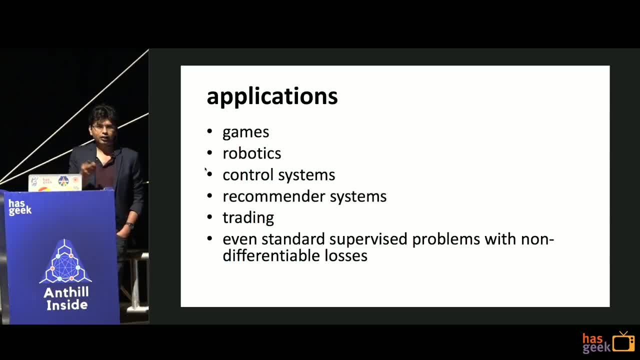 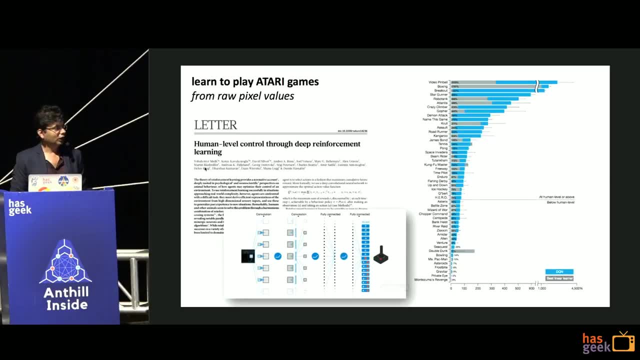 own setup, whatever problem you have. how do you formulate in that? And then there are certain standard algorithms which you can to crank the machinery. So I will just briefly flash a couple of examples before we get into the details. So let us start with the first example. So this was in 2013, I guess, where deep mind showed that. 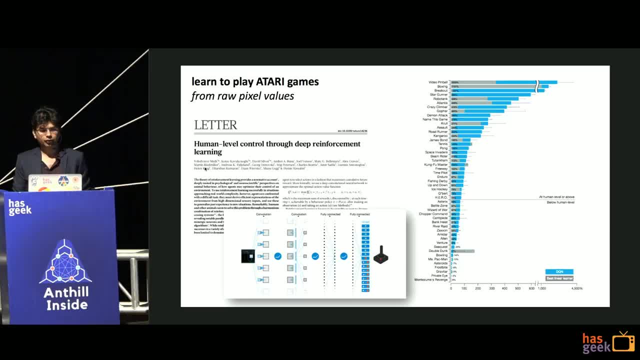 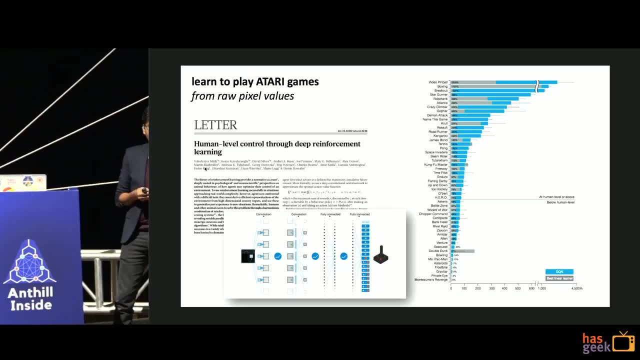 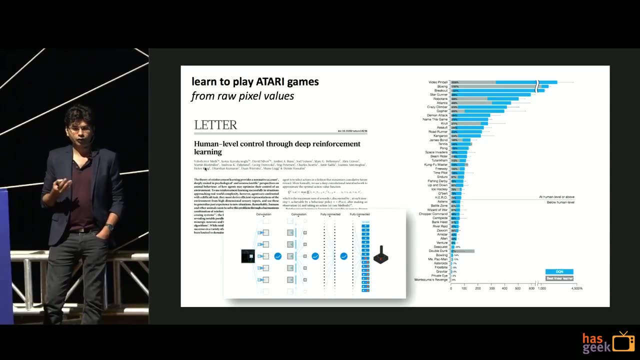 you can actually learn to play Atari games just from raw pixel violence, right? So the examples I am showing are some kind of success stories in deep reinforcement learning rather than reinforcement learning. So reinforcement learning has been there for quite a long time, but it was not successful, mainly because of this. still, deep learning came in, because 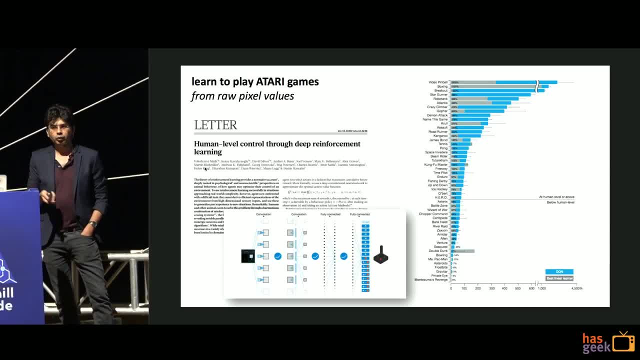 of this infinite state space. There are lot of computational issues, But after a couple of these since 2012-13, there has been kind of a tremendous progress in deep reinforcement learning. yeah, So probably, I think. just let me just make a comment. I think these are: 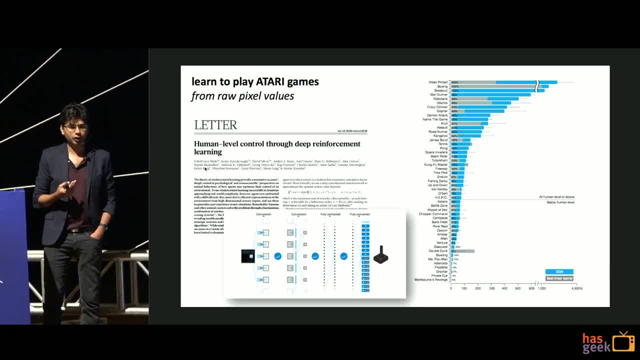 the two talks the way I have arranged. I think these are probably currently the most hot areas in deep learning. One is the deep reinforcement learning and after this, the second talk, which would be the GANs right Probably. that is why I think you can see, probably if these 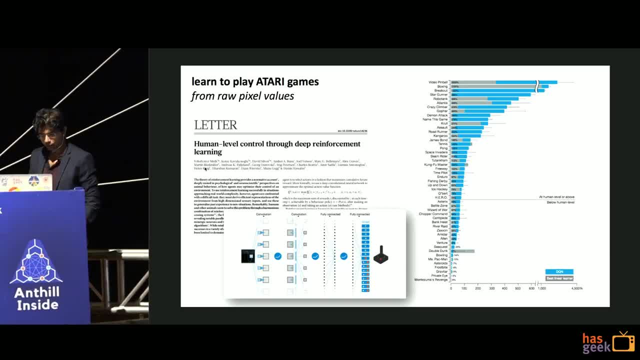 are almost on the cutting edge of the currently the deep learning setup. yeah So the at least. yeah so the. what I in this, what I want to point out, is that to learn this, all you need is just the pixel value right of the Atari game, and they were able to figure out how. 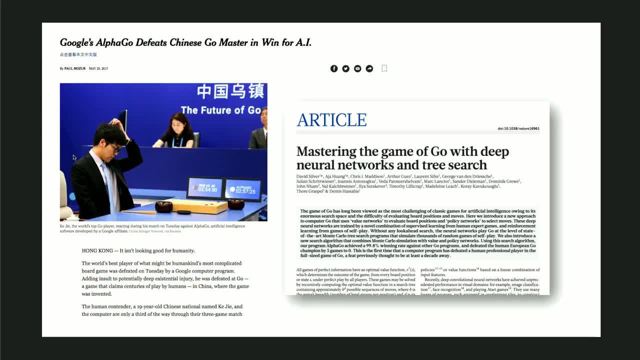 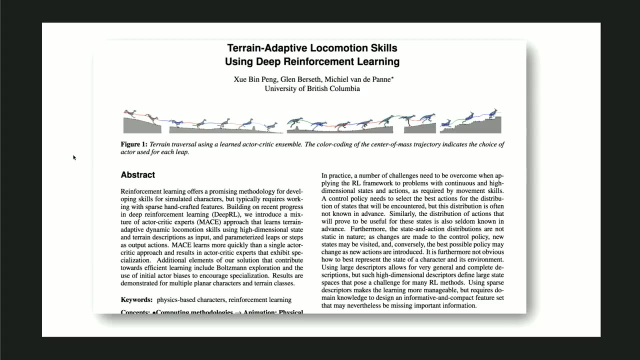 to play the game. yeah, Then the Google's alpha go, which defeated the go was essential. another in- I think this was in 2017, right, This was again purely based on kind of the deep reinforcement learning framework Then. so there are other examples, lot of examples in robotics, right. 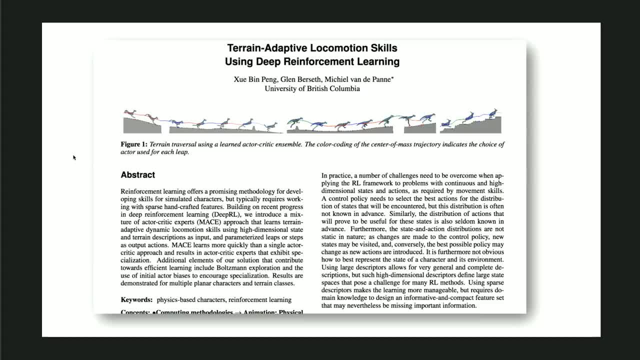 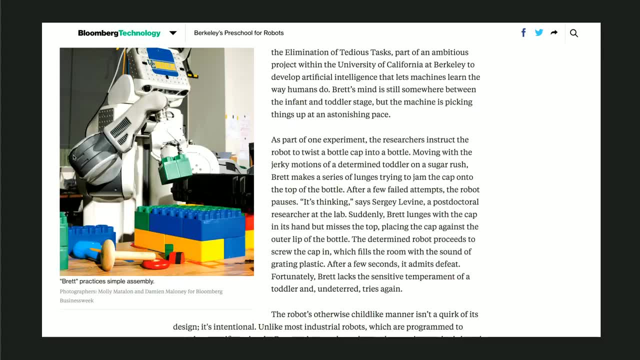 How do you make a creature jump in a terrain? How do you try to control it? Those are kind of lot of examples coming up in robotics And this is an example. in Berkeley there is something called as a pre-school for robots, right, Essentially the way humans like kids. 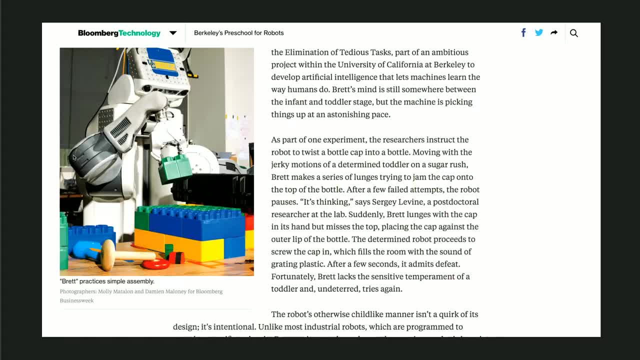 go to pre-school. you can have like robots go to pre-school where they just keep trying learning things And essentially the whole loop- the closed form loop- is a reinforcement learning loop where they keep trying: how do I lift here and keep it there? How do I grasp? 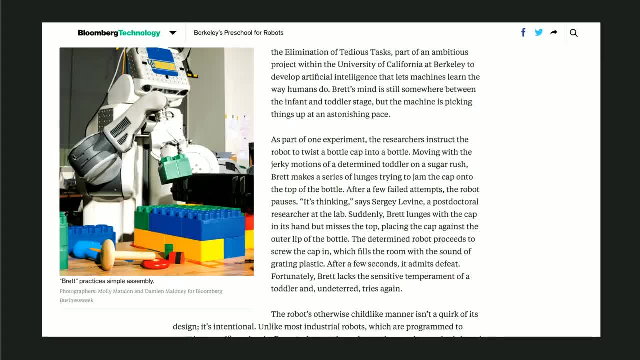 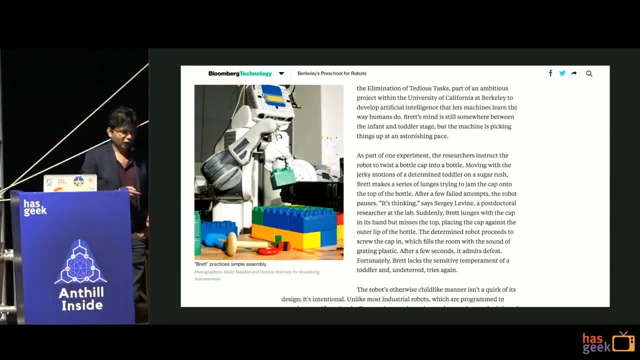 something, yeah, And essentially they are just sitting and trying and doing that for days together. That is essentially, but we will come to the formalism later. but that is one example to think of. So I will also give you one example in a recommended system, and this is exactly also what I am. 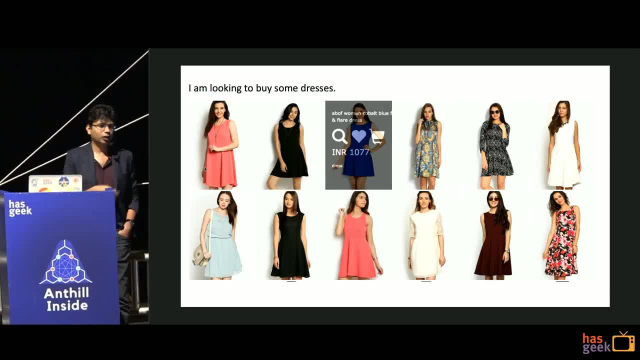 trying to. this is some work going on in our labs which I am trying to cast even a recommended system as a deep reinforcement learning program. Say, for example: you say I am looking to buy some dresses. You get some items in the catalog. Then you say the user actually clicks on a. 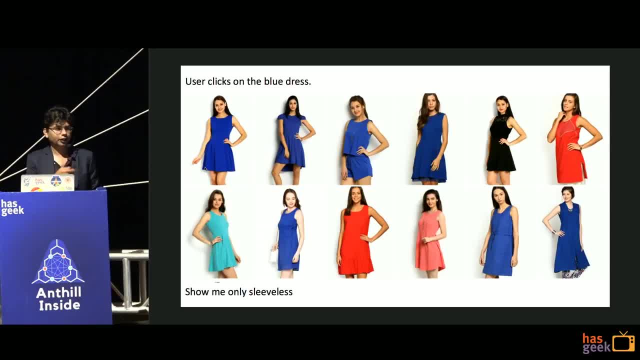 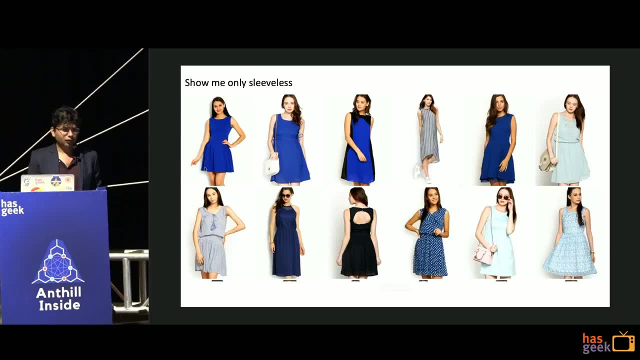 blue dress, Then it shows some blue dresses, Then again the user converses: say show me only sleeveless. Then again it picks up sleeveless dresses, etcetera. yeah, So this is a kind of: you are interacting with the catalog, You are making some actions, The system is showing 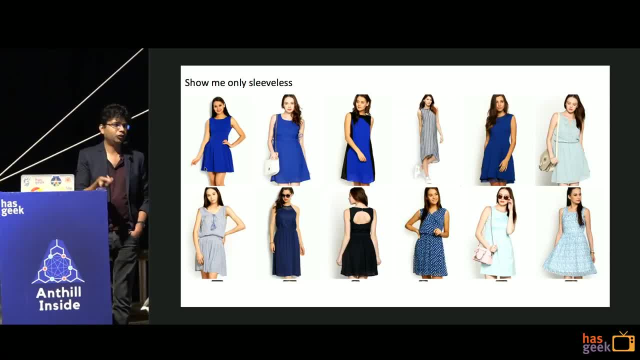 you some results and you are getting a reward in the end. What is the reward? Someone adds that item to your cart right Again. how do you formulate will come to that? but again, this sort of simple multimodal conversation system or learning your recommendations can. 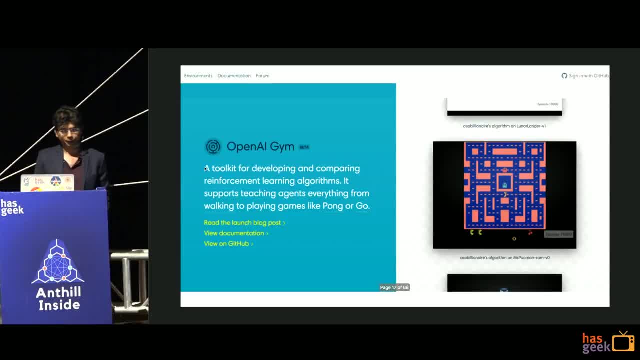 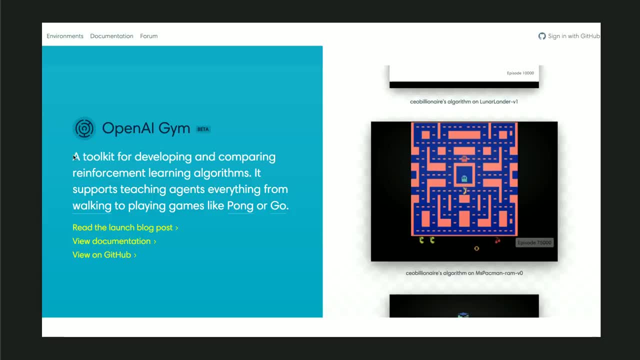 itself also be cast as a deep reinforcement learning program. yeah, So I will also point out to this thing side called as open AI gym, which is essentially lot of these examples which are pocket water coming from there, which is essentially a series of video games. 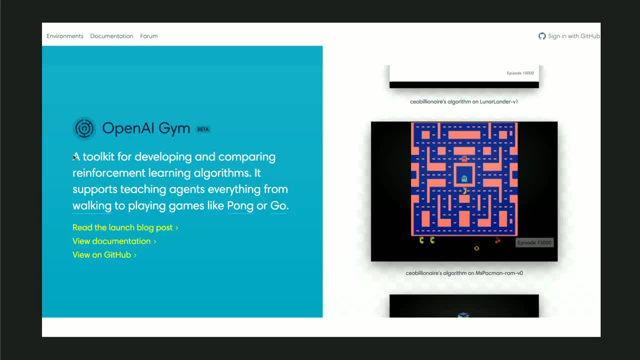 You can think of it as more of an test bed to test your deep reinforcement learning algorithm, right? So you will get an example of some game where there is some AI agent which is one side and you are trying to your reinforcement learning algorithm to kind of win the game. yeah, So there? 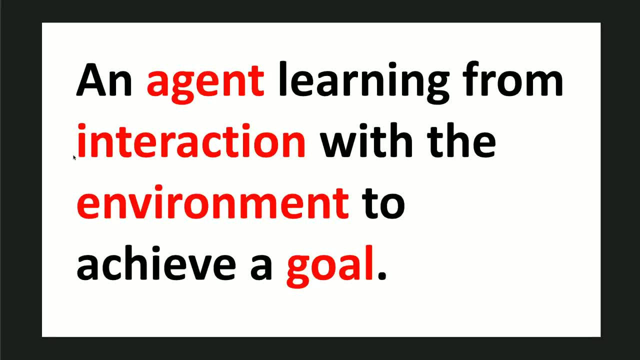 are a lot of games in there. Okay, so that is the introduction. Now I think we want to do a deep dive into the deep reinforcement learning framework. yeah, So I will again come back to the formalism, which is an agent learning from interaction with the environment to achieve a goal. 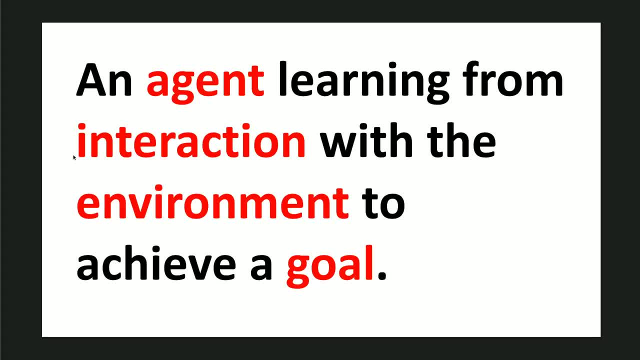 yeah, And this is what we want to formalize: What is an agent, What is an environment? What do you mean by an interaction And what is the goal and how do you achieve that? So, as I said earlier, so this kind of, there is this whole concept of supervised learning. 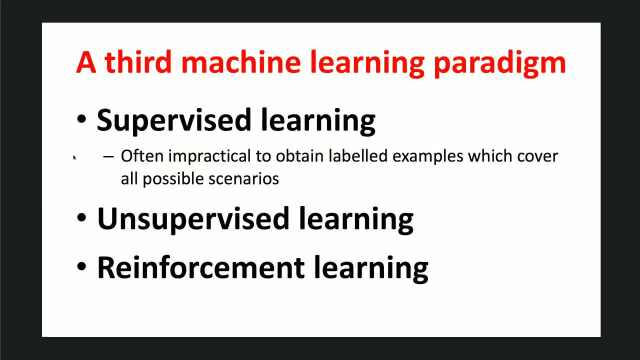 where you are given explicit labeled examples to learn. Then there is Unsupervised learning and what we are talking about, the third paradigm, which is called the reinforcement learning, where in lot of examples it is often impractical to obtain labeled examples which cover all possible scenarios. That is why it is a very natural way to kind of formulate: 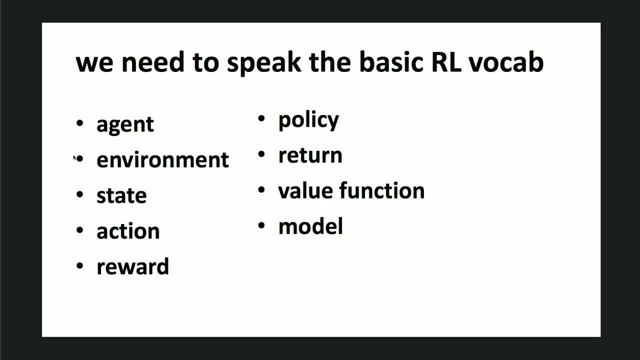 problems in the reinforcement learning center. yeah So, before we even understand deep learning, we need to need to speak the jargon of deep learning right? If there are, I mean if you, if you think these are all very familiar, then please raise your hands. then I would not cover. 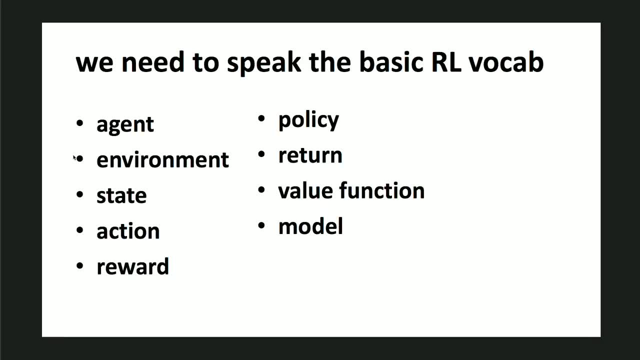 but this is exactly what we are trying to cover, right? What is an agent, Environment, state action, reward policy, return value, function, model, right, These things, any problem you think of, if you can actually map your things to these. 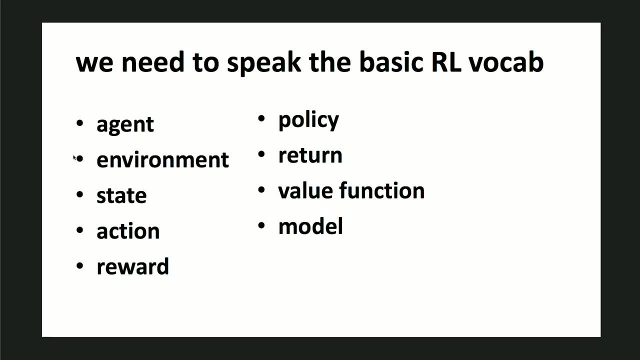 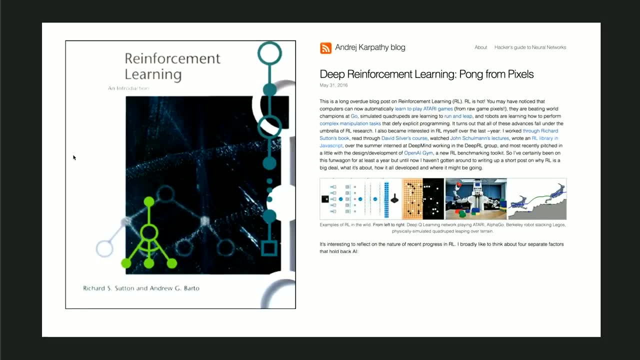 things. then you know how to cast a problem in RL framework, yeah, But so we will just go one by one and that is essentially the main one. yeah, So my references for these are two things where I prepared the talk. So one is this: Richard Sutton's book on reinforcement learning. There is a new. 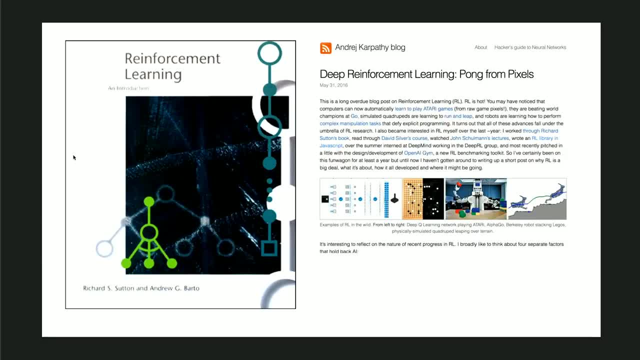 edition. I think the book is pretty old now, So he is writing a second edition of the book that is freely available online. and you want to go deep? chapter one, two, one, two, three are the things where you will get a good sense of reinforcement, learning right. But after one, two, three, you 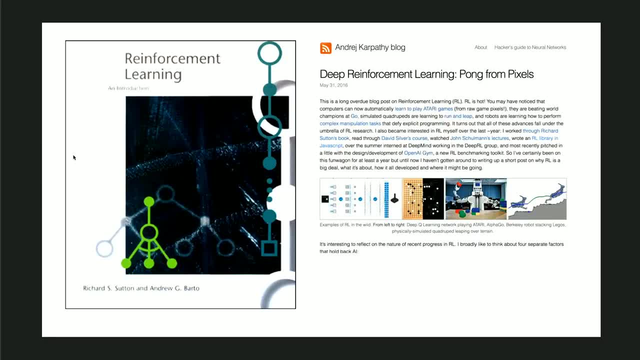 can actually stop after that. it is all classical reinforcement learning. Then you probably deep reinforcement learning hardly. there are not many textbooks out there yet, But kind of the example I am taking is from this but Carpathi's blog on the deep reinforcement learning. That is the working. 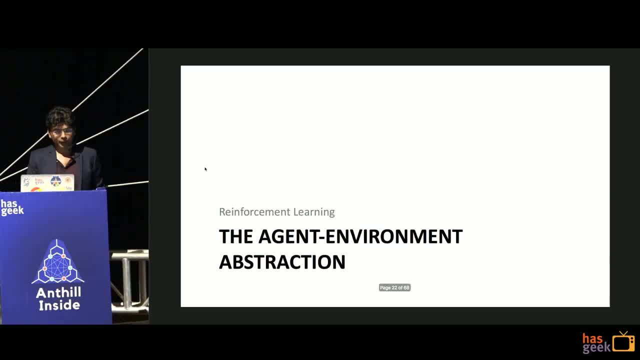 example I am using. So I am going to show you how to do that. I am going to show you how to do that. Okay, So let us dig deep now. yeah, So essentially, we are trying to formulate this: agent, environment interaction. yeah, So, again, we will reiterate the same thing. So an RL agent must be able to do three. 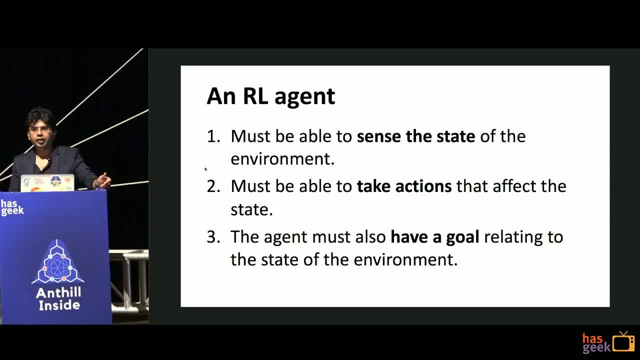 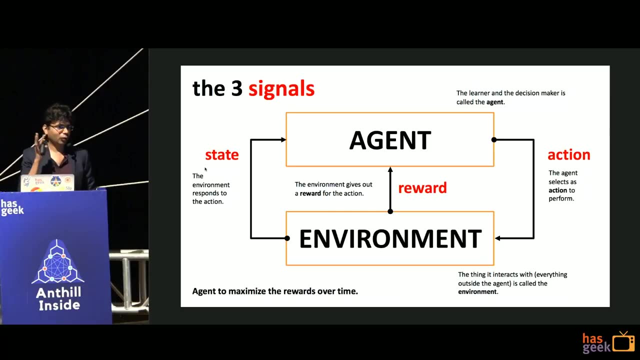 things: It must be able to sense the state of the environment. yeah, It must be able to take actions that affect the state. and the third one: the agent must also have a goal relating to the state of the environment. So this is the diagram, I think. probably try to memorize, right. This is what 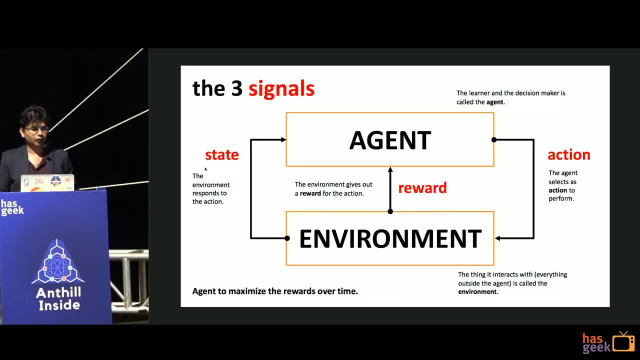 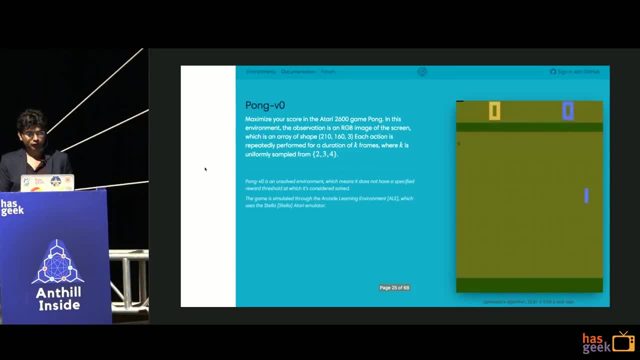 we will have to keep using back and forth again. yeah, So there is three things here, So the agent and the environment. yeah, So the agent is the learner and the decision maker is called the agent. Can I have an example? Okay, And the environment is the thing it interacts with is called the. 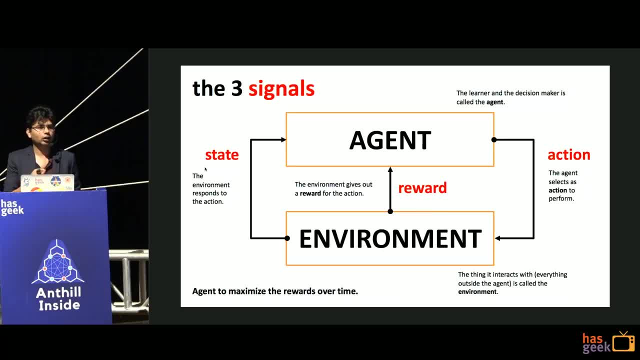 environment. So an agent is someone you are trying to learn right, An RL agent, some trying to make the action. Environment is something which is completely outside the agent. that is how you think of the environment. So the boundaries are all dependent upon the problem. It. 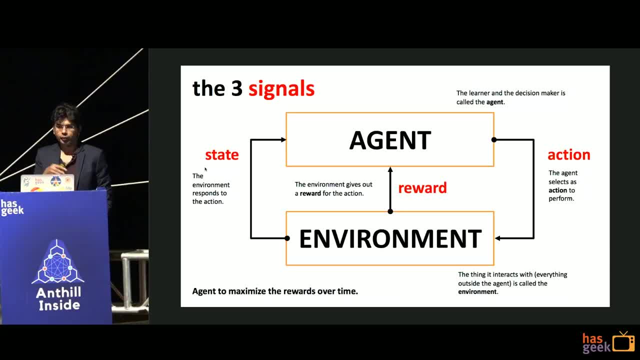 does not necessarily mean that the environment and agent can also be the same person, or it can be the same robot. Essentially, where you demark it, I have to take an action. Whatever is outside the agent is environment. yeah, So the agent actually takes an action. yeah, The agent selects an action to. 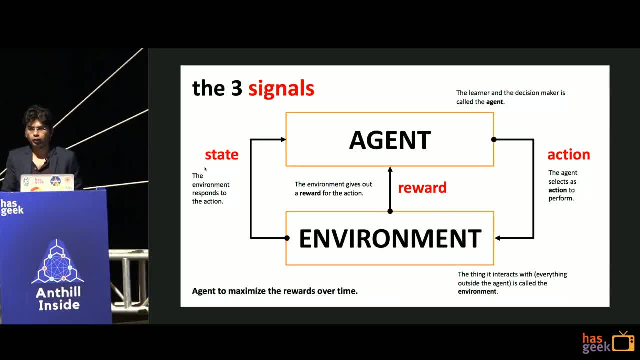 perform. yeah, It could be here that I am trying to get up or trying to walk, right, That is an action. So the environment actually gives out a reward for the action. right, You take an action, take some action, and you get a reward out, And the state is essentially once you get that reward. 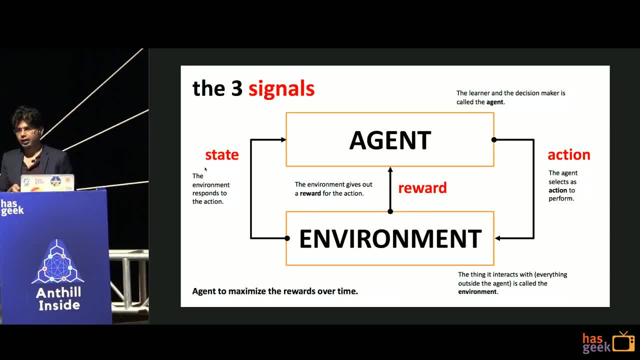 the state gets modified. yeah, So I will come. we will again reiterate these three things, But things you need to remember are action, reward and state. So the agent takes an action, the environment gives you a reward. Based on that, the state changes. 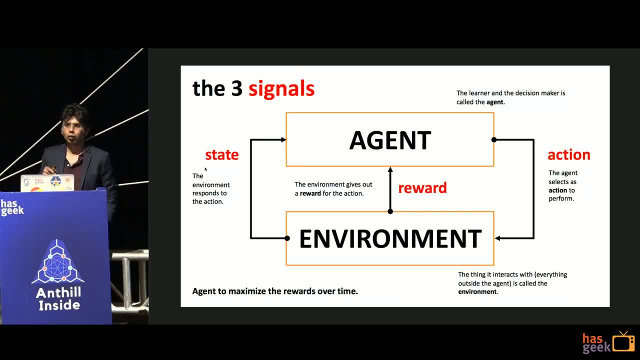 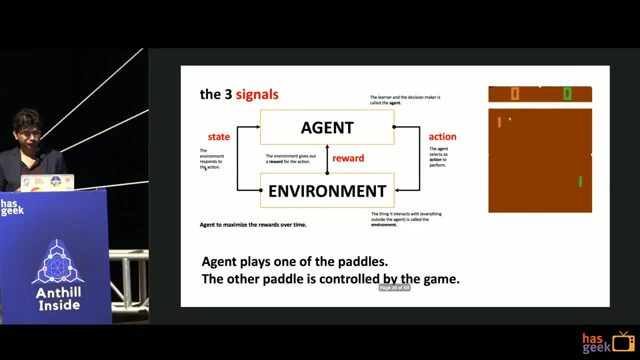 Then again the agent takes the next action, and this is a control loop or this is a closed form loop that keeps continuing. yeah, That is the basic formalism of an RL problem, So we are going to use this example throughout. yeah, So this is what is called as the one of the. 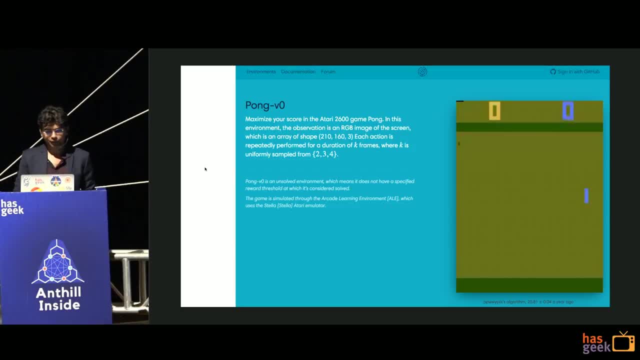 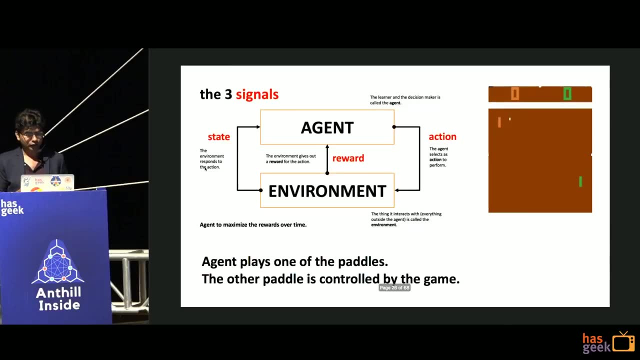 games in the open gym. It is called the Pong game, yeah, So let us spend some time on what is that we are trying to do here. yeah, There is a video here, but it does not work, So let me just directly. 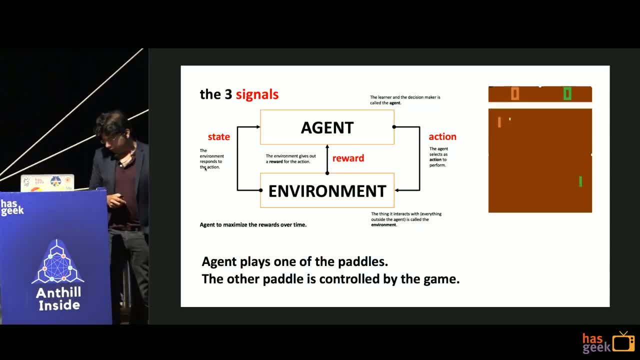 go to this part. yeah, So this is think of this as a classical ping pong, right? whatever your table tennis. So what? you see that there are two paddles here. Let me see. yeah, So this is, this is one paddle here. There is another paddle, These are two ping pong pads, yeah. 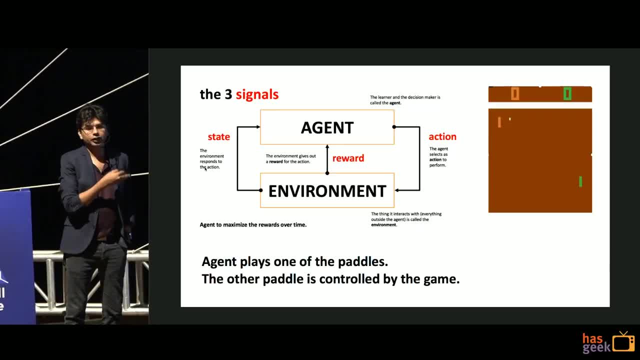 So this paddle is controlled by an AI agent. That is essentially the game. who is controlling it? yeah, And this is you are playing this paddle. yeah, So your goal is essentially you can move the paddle up, down, etc. And there is the ball here. yeah, So you essentially take this paddle. 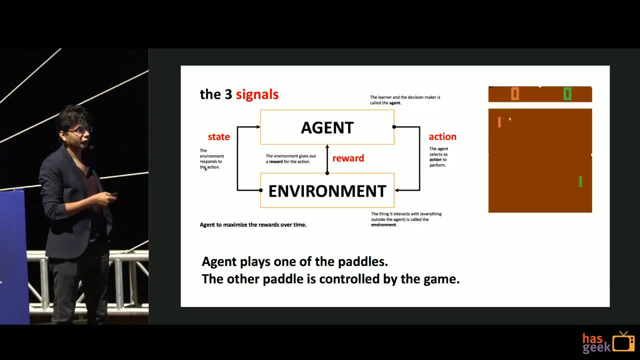 hit the ball and it goes up here and then this guy hits back and that is how you play the game. You are essentially playing a ping pong on this grid of, say, 200 cross 100 pixels. yeah, And every time say you, you hit this ball. let us say the AI agent or the other, the play the game cannot. 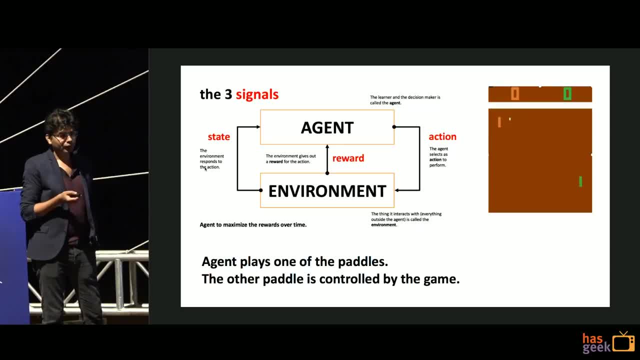 intercept it and it goes out of the boundary, then you win. yeah, So you if kind of the, or if you essentially this guy hits it and it goes out and you cannot intercept it, then you lose. yeah, So if you hit once, you get a reward of 1, or think of you lose, you get a reward of 0.. 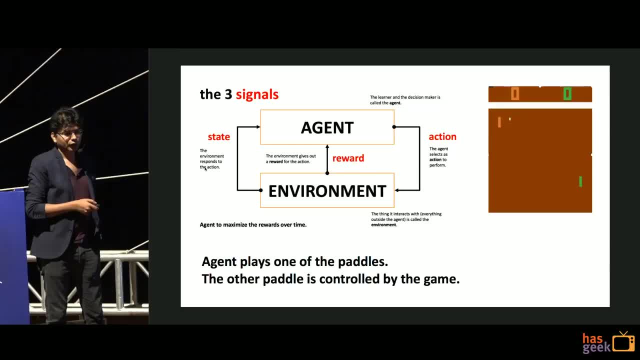 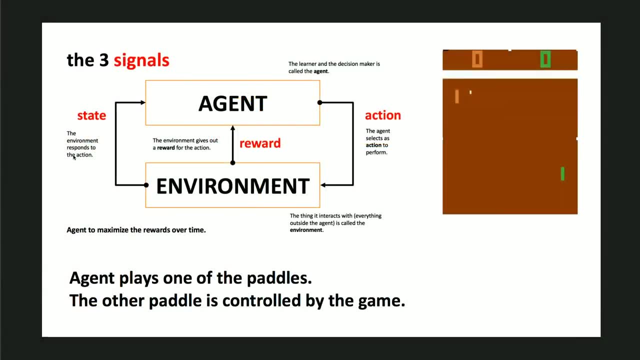 So essentially, there is a counter here which says how many wins you get right And that is how the ball goes in. So essentially, classically, it is just a TT game, table tennis game. right, You are just passing the balls anywhere And the only what the goal here is that I need to figure out. 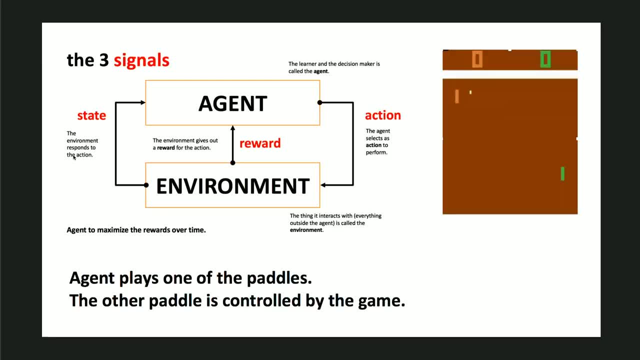 how should I hit? yeah, So the green guy. what you see, right, that is the RL agent. So I am going to play this game for many times, many, many, 100,000,, 1000 times, and figure out how to game play this. 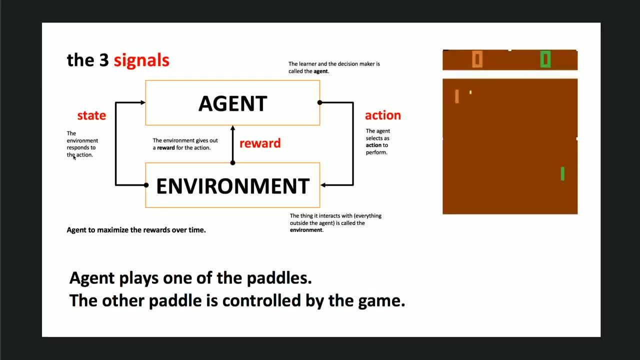 game perfectly right, without any supervision. yeah, No one is going to tell me how to play the game. right, You have the game engine, which is you are playing with. Think you think that you are going to play with an opponent? yeah, And so you are going to play with an opponent. right And so. 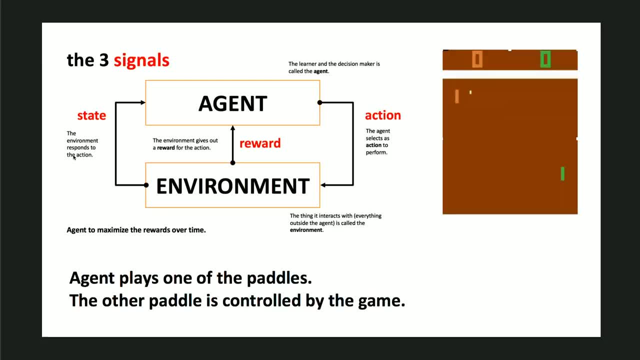 now you are going to play around and then figure out how I am going to win. yeah, So that is the set up. So that set up is pretty clear, right? So the issues on that. okay, So the agent plays one of the paddles and the other paddle is controlled by the game And your goal is: 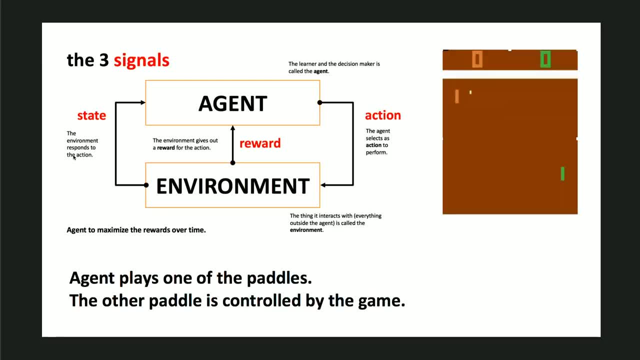 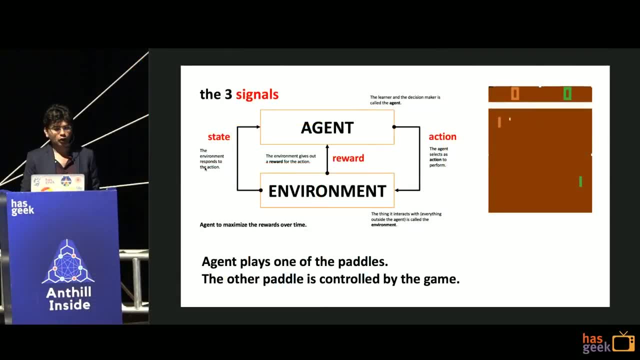 actually to learn how to play the game. yeah, So that is the reinforcement learning framework. Let me just briefly mention one point that if you want to learn this right, the AI engine, which is the orange one, it cannot be a perfect engine, right? If it is a perfect engine, that means that 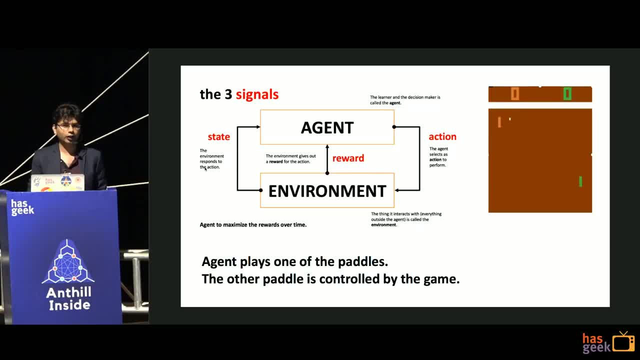 you are never going to win and you are never going to get any feedback on what kind of actions do I need to make to win. So, typically, generally, this game system is also an imperfect AI system. right? So you are actually. you have some chance of winning, but you are going to play around to. 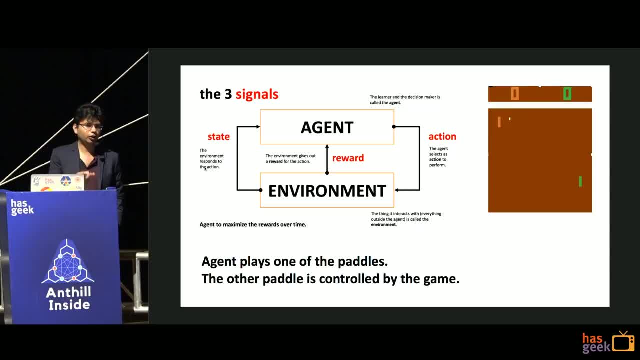 figure out how to win and lose. So you are going to start playing, You are going to win some, You are going to lose some And eventually you want to learn a policy or a strategy: how I am going to win against the opponent. yeah, If the opponent is perfect, there is nothing. I mean you will. 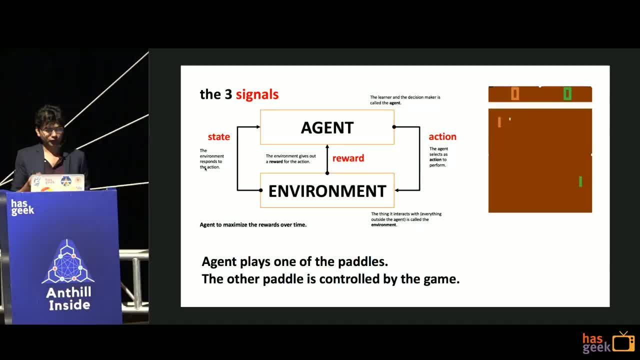 probably you will not even get a chance to learn anything, yeah, unless he explains it. So that is the game system, right, You have some chances of winning, but you are not going to play around to unless he explicitly teaches you. Okay, So, so in this context, okay, so I will tell coming. 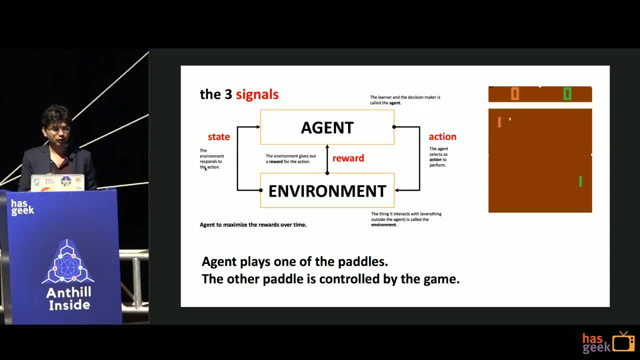 again, What is the agent? Agent is the green paddle. yeah. What is the environment? Everything other than the green paddle, The entire array of the whole game. that is your environment. What is your action? I can take either the paddle up or down, right. Essentially, I am. 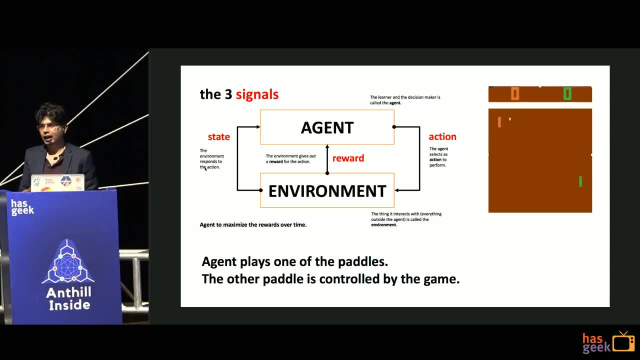 moving paddle up and down to intercept the ball. That is why that is the action. So what is the reward? Either I win the game, I lose the game or nothing happens, because I get is just in some state of the game And what is the next state State is essentially 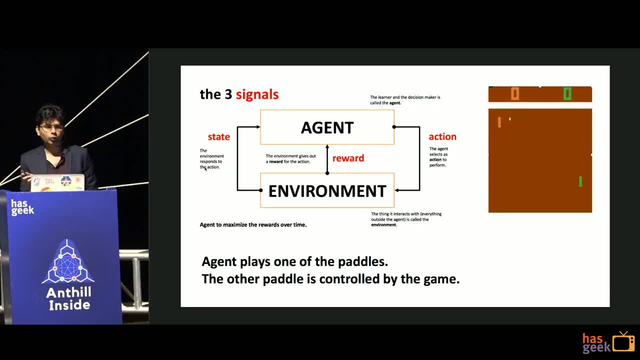 the whole image right? So you, you get the ball at green, you give one smash, it goes around and then you get some reward and after that the state changes, which is essentially the new position of the ball. yeah, So that is how you abstract this problem. in this sense, 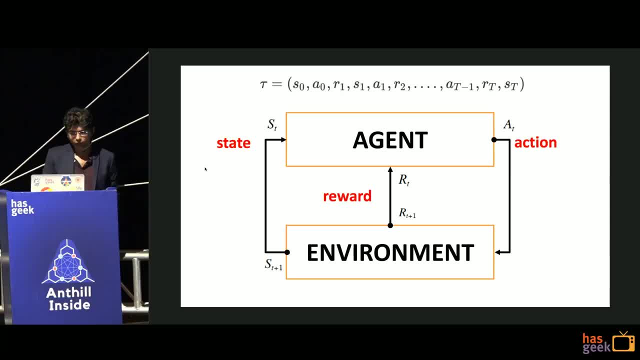 So now we will start introducing little bit more notation. yeah, So we call the action as an AT. yeah, We call the state ST and a reward RT. yeah, And a game essentially is a sequence of this. right, You start with state S- naught, you get an action. A naught, you get a reward R. 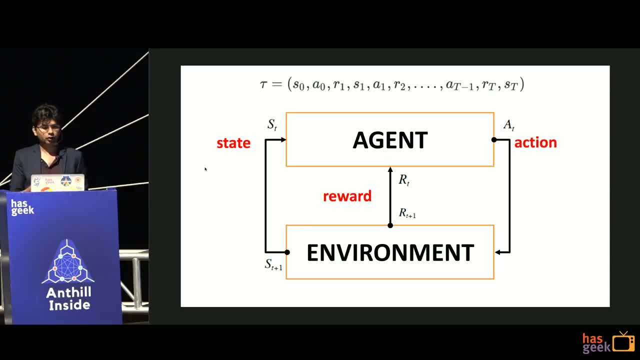 1, state changes to S 1, you take an action- A 1, you get a reward- R 2, you keep continuing till you hit a terminal state. And what is the terminal state? You either win or you lose. At that point, you stop, the game restarts, you continue. yeah, That is essentially how. you are playing the game And this is a mathematical argument. yeah, So you start with the state S: naught, you get an action A. naught, you get a reward: R 1,. state changes to S 1, you take an action A. naught, you get a reward, R 2, and you play with the state S naught. So you are passing a kind of a game on A naught. So any number of states becomes a kind of a game after you have used a particular state. 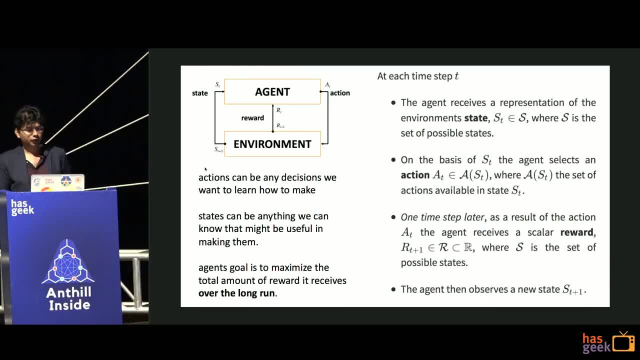 Now, what is a state, A naught? A naught is a time stage. A naught is a time stage, So you can now take that general judgement of any time state. So here A naught is a time stage where a state is two points. 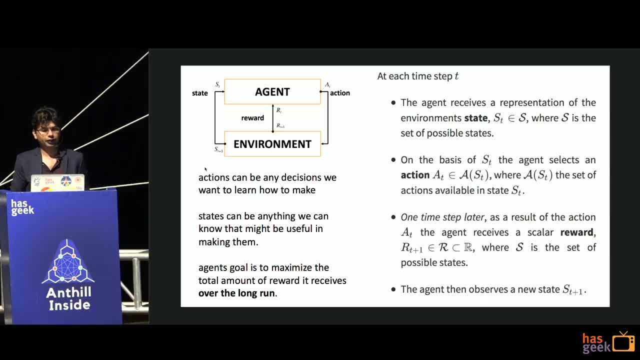 So you can connect one point to the other point and the other point to the other point. Here A naught is a time stage, So you connect an action A naught to the other point And this is how we call state as an action A naught. 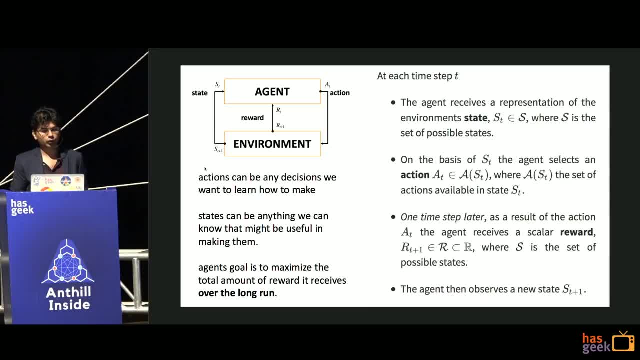 So you connect a action A naught by a time state. The agent receives a representation of the environment, which we call the state ST. yeah, state S belongs to this capital S, which is the set of all possible states. On the basis of S? t, the agent selects an action A t which is also belongs to some space, One time step. 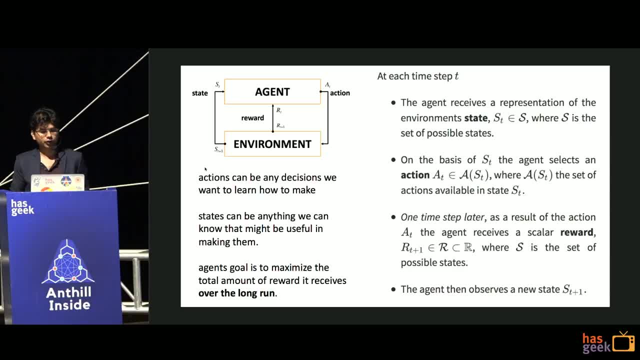 later, as a result of the action, the agent receives a scalar reward: R t plus 1. Again. so this is a little bit. if you look at the literature, there is some confusion between R? t and R? t plus 1, but I prefer this notation. where you get S? t, you make an action, A t after. 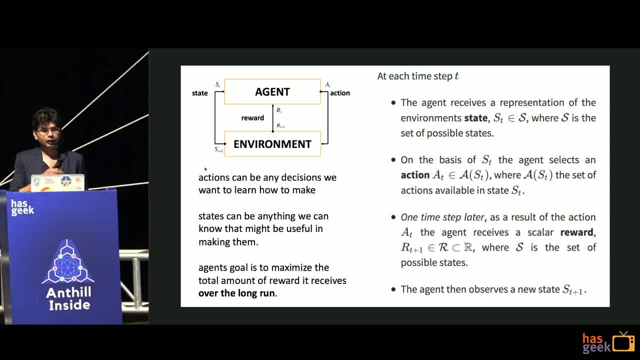 one time step. you get a reward- R t plus 1- and then the state of the system changes to S? t plus 1. yeah, So that is the closed form loop. yeah, So little bit on how we want to do is actions. again, to generalize this, actions can be any decisions you want to learn to. 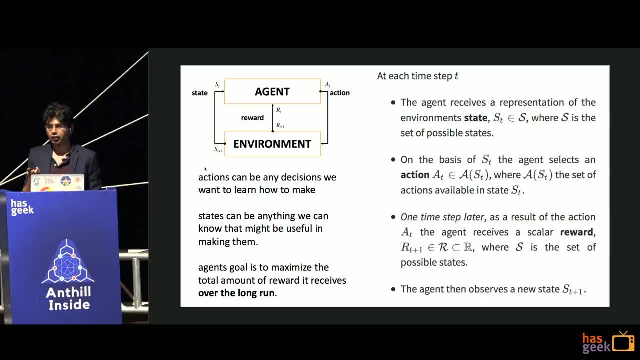 make right. So anytime you think about problem you need to think: what is the action right? what is my action Here? the action is very simple. I move the paddle up, I move the paddle down, Okay, and state what is state. State can be abstracted by anything you think the action. 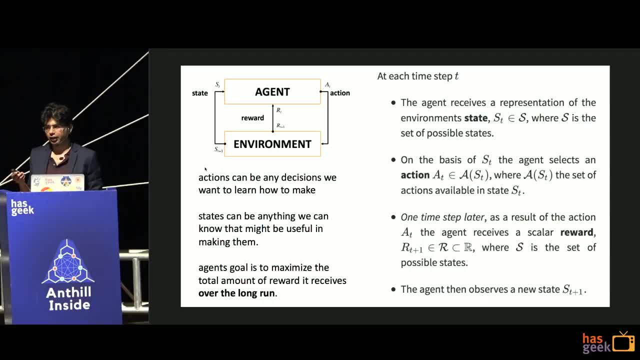 has to be influenced by. It does not have to be a perfect everything right. It can be a simple thing. what p set of features you think will be responsible for the action? right, It is all the game of how you model your state. yeah, And in the end, the agent's goal is actually. 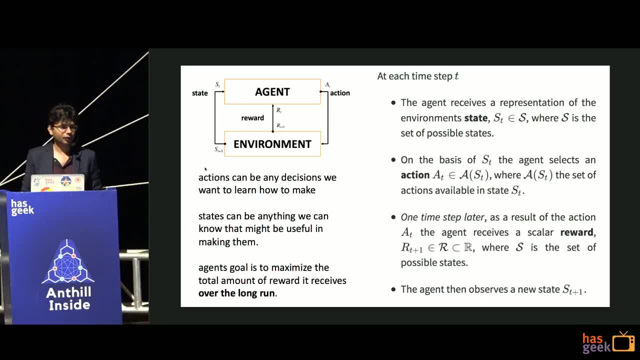 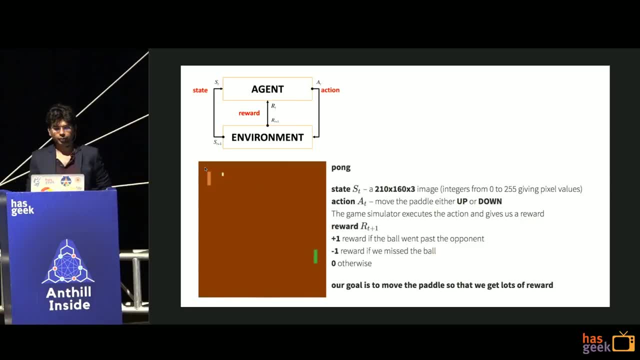 to maximize the total amount of reward it receives over the long run. yeah, But I have not formalized this statement yet. that is what we will do in the next couple of slides. So again we will come to this Pong example, right? So what is state now? more precisely, state is nothing but this: 210 cross, 160 cross 3. 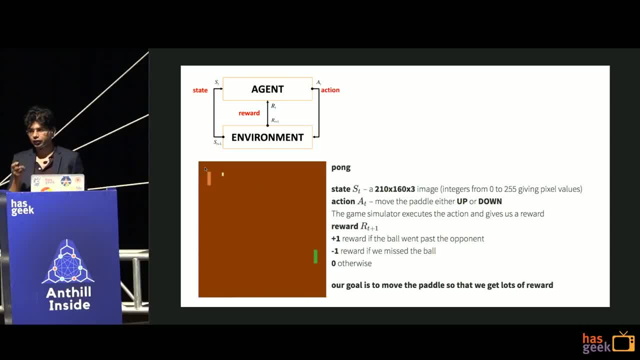 R pulse. Again, this is how we will be, where each pixel in the image is some number between 0 to 255.. So think, as this roughly 100,000, 800 numbers is your state- yeah, which is what you want to do, Your state is a vector of 100,000 dimensions, which is- I just flattened this- 200 cross 210. 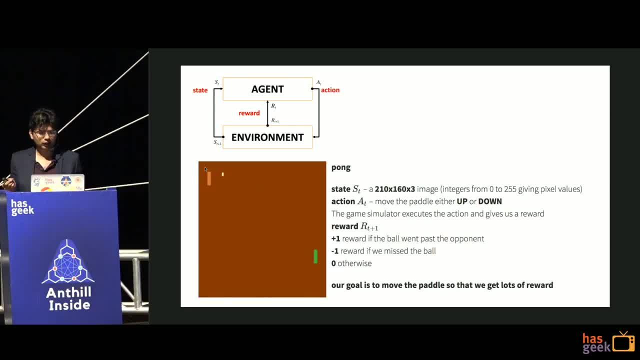 cross 160, cross 3 image into a long 25.. Okay, that is the end. I did not want you to fail, I did. just saw the other side of that before itself, That's, if you can see the paper which doesn't match every other capital here, Then treat it. 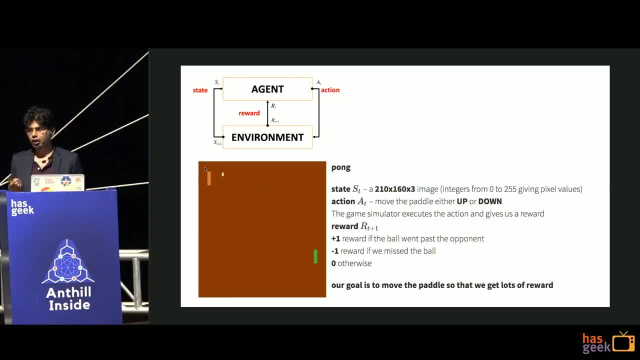 What is action? Action is either binary, up or down. right, There are only two possible states. And what is the reward? Reward can be three things: Plus one if the ball went past the opponent, Minus one if we missed the ball, And zero otherwise- Zero, most. 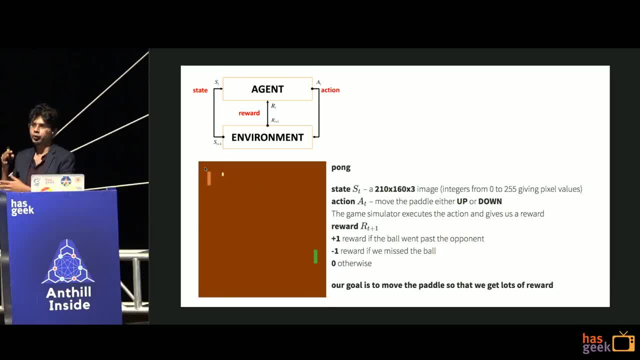 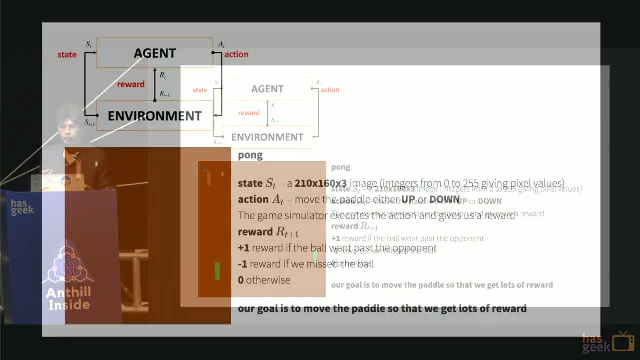 of the time you are playing, it will be zero right, Because nothing is happening, But only at certain points. you either win or lose, And that is when you get the reward right. And the whole point is to figure out: how do I get this? plus ones, a lot. That is essential. 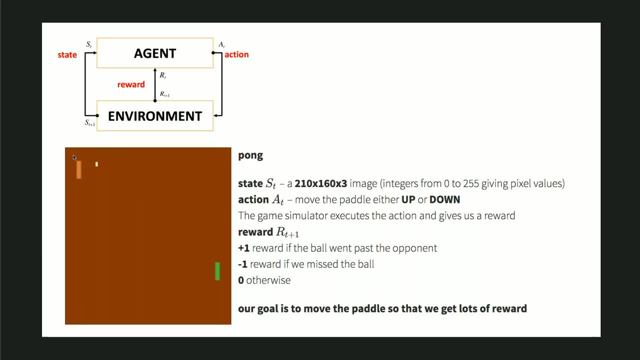 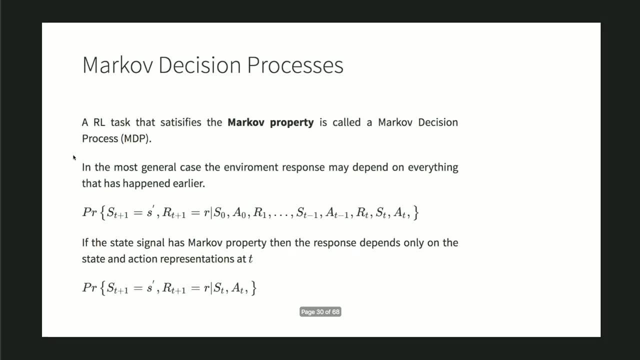 So your goal is essentially to move the, decide how should I move the paddle up and down based on what I see in the image, So that I get lots and lots of reward? okay, So before I move into something, I will just briefly something formalism called. so you 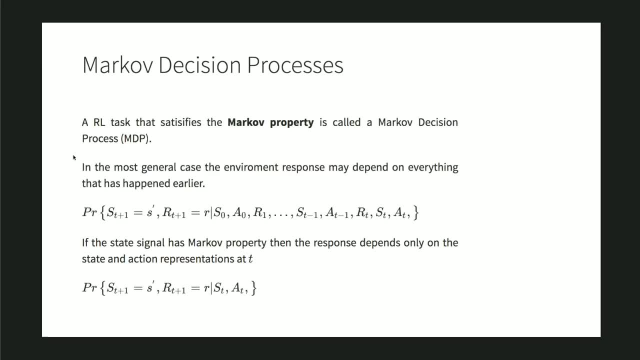 probably have heard the term Markov decision process, And Markov decision process, or MDP, is another ERL task with a certain special property called the Markov property. yeah, So what does it say? So this is essentially a way of. 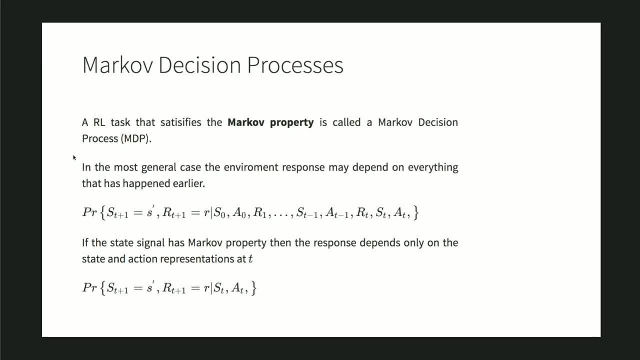 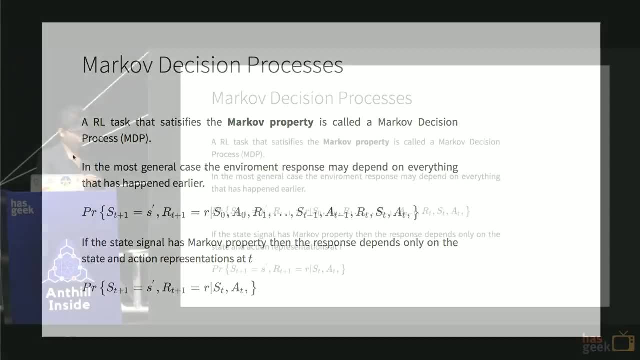 kind of simplifying our state dynamics. So what does that mean? That I take some action, I get a reward. my state changes, right. Something happens to the state, which is essentially what I am showing you here, right? So ST plus one is a new state, RT plus one is a. 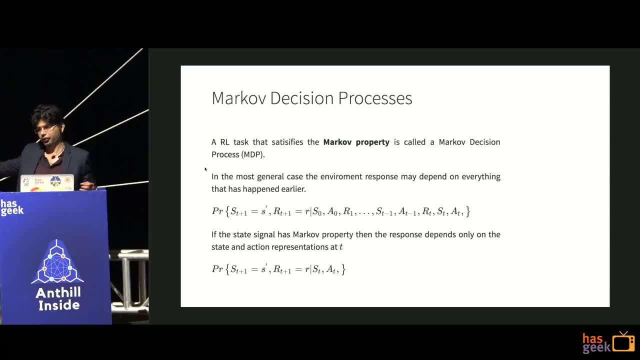 new reward. In principle, this change can depend upon the entire history. right, You can go all the way back to your game or whatever, everything it can depend, right? So Markov assumption states that it depends only on two things. right, Which is essentially your. 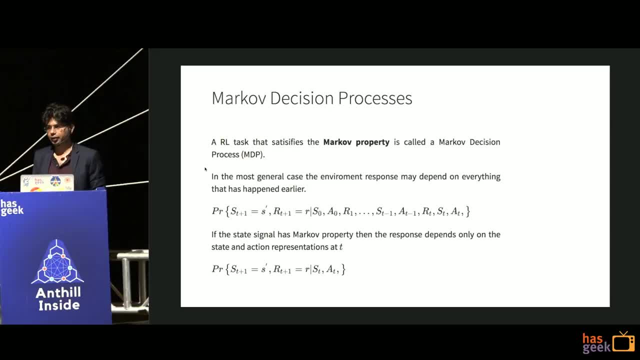 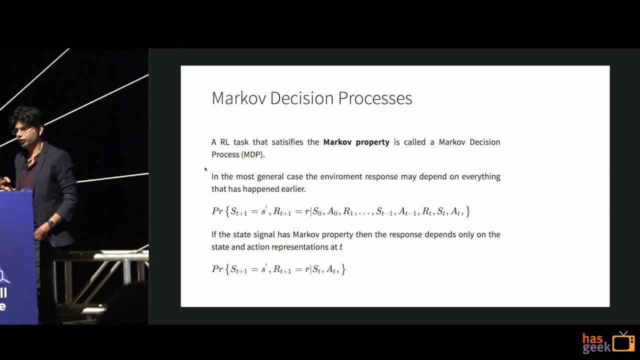 previous history, which is ST and AT The last, two things right. So the first thing here. So the one example which I always I find it very interesting, I think, is think of playing the game of chess. right, So it is. chess is again a classic. you can formulate: 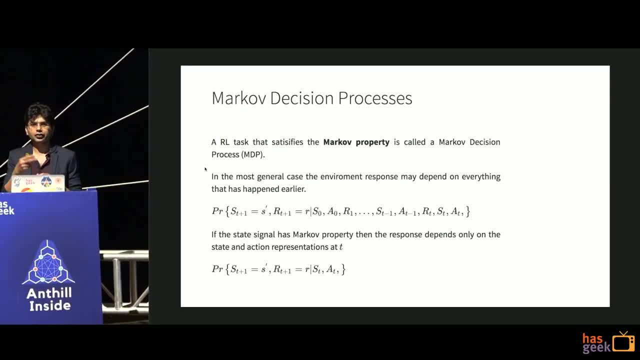 it in RL framework, But any time you want to make the next state, so you all that you can do is depends upon the current state of the board, right? You do not have to know how you came to that board, right? It really does not matter whether you took an action. 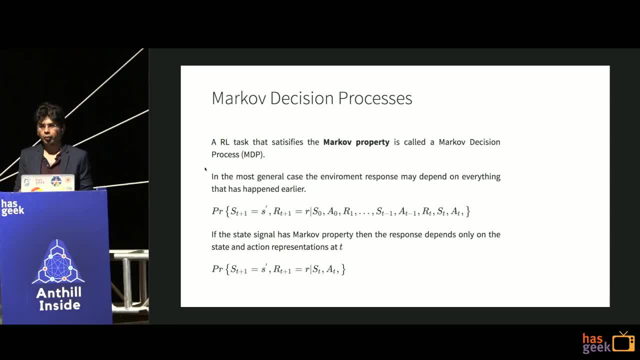 from there you took. there are multiple ways of coming to that state, But once you are in that state, that is all it matters. Based on that, I can figure out what should be the next action. So that is the next step. So that is the next step. So that is the next. 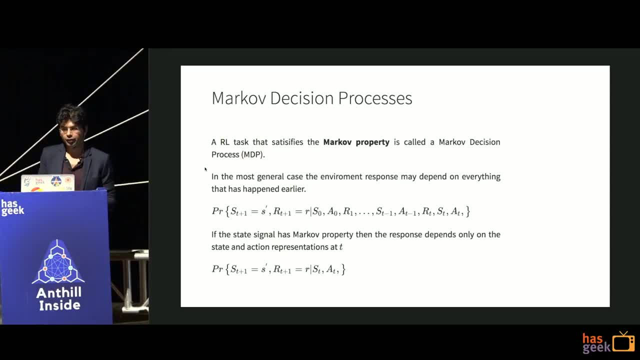 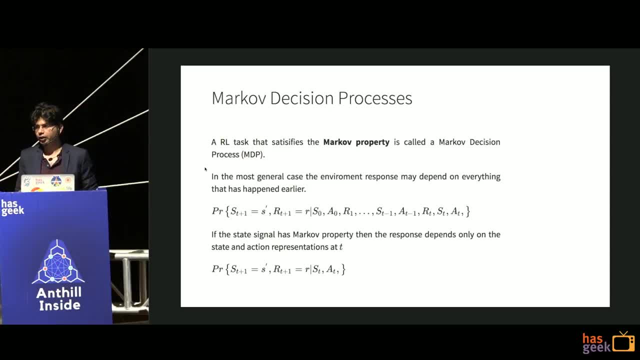 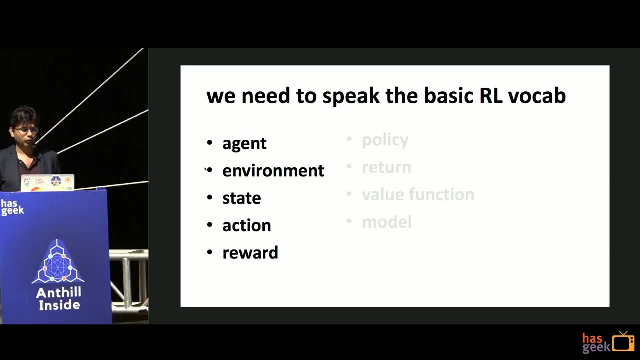 this is the Markov assumption. yeah, Even though the Markov assumption may not be true, it it makes sense to actually, ok, actually formulate: this is the Markov decision process, yeah, OK. So now coming to the, we need to speak the basic RL vocab So we know what. 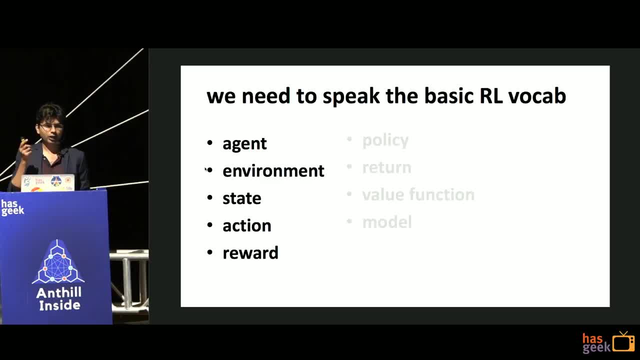 is an agent. we know what is an environment. agent is the paddle and p Model is L is the environment, is your entire grid state is actually the pixel values. action is: move the paddle up and down. reward is plus one, zero minus one. yeah, that's the reward you get. so now we come to the other. 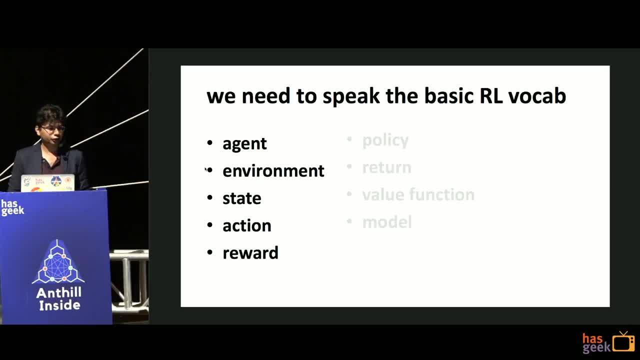 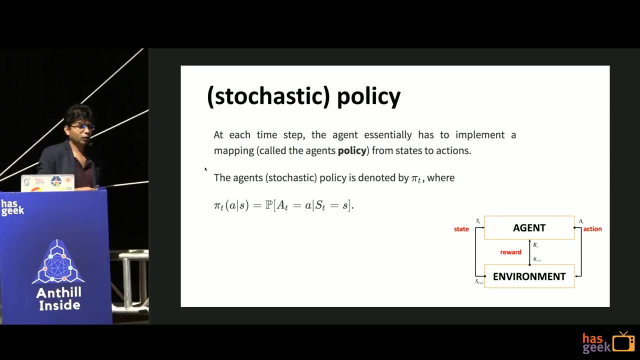 four things, which are policy, return value, function and model. yeah, so once i get these four things, i think you'll have a clean understanding of what is the reinforcement learning problem. okay, so we now come to something called as a policy. so, at a high level, policy is something. 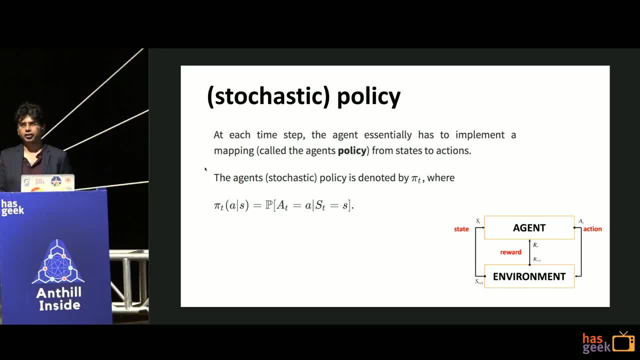 what is the action you want to do here? i mean abstractly, what is it? i want to decide whether i want to move the paddle up or paddle down, but at each step the agent has to implement a mapping from state to an action. right, given a state, that is the pixel. given this current air, how, the current 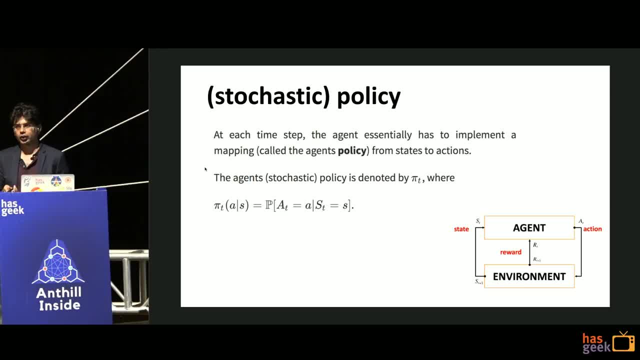 state of the game is. i want to decide what should be the action i need to take. either should i move up or not. that formalism, the way of mathematically writing that is called a policy, which is what we use. the notation pi of a given x, given that i am in state, is: what is the probability that i will? 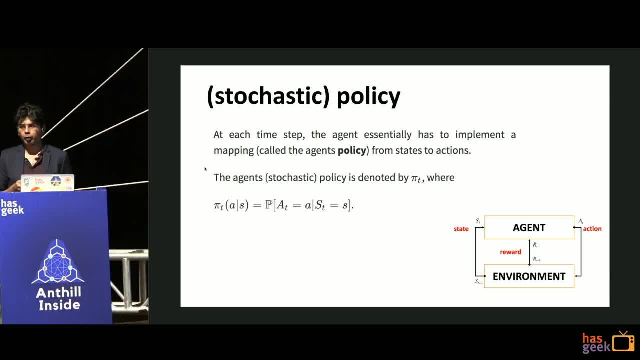 take an action in? yeah, given that this image, what is the probability that i will move up, or what is the probability that i will move down? yeah, so most of the deep reinforcement learning will use this notion of something called stochastic policy right, which is essentially you, rather than taking a. 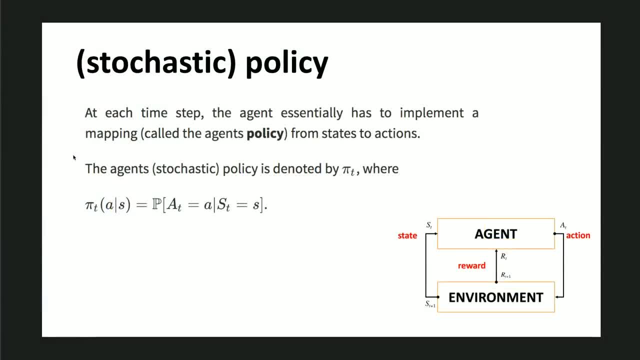 deterministic policy, whether i can move up or down. all this compute is some kind of what is the probability that i should move up, what is the probability that i should move down? and you start sampling for it, right? so if you say probability of going up is 0.9, going down is 0.1, you actually toss a biased point in probability 0.1 if it is. 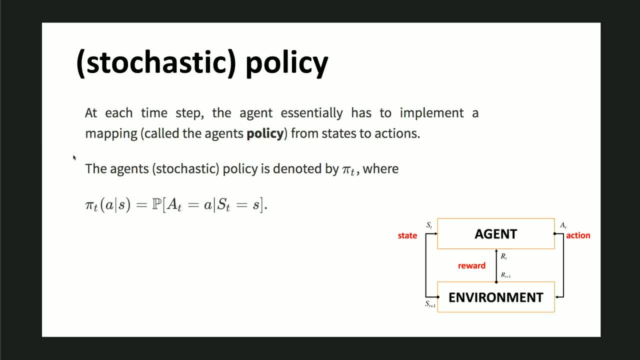 that you take that action, otherwise you go right and it's very. it actually looks very simple, but there's a very strong reason why you want to use stochastic policies: because you want to encourage a lot of exploration. so if you don't use stochastic policy, you're always taking the 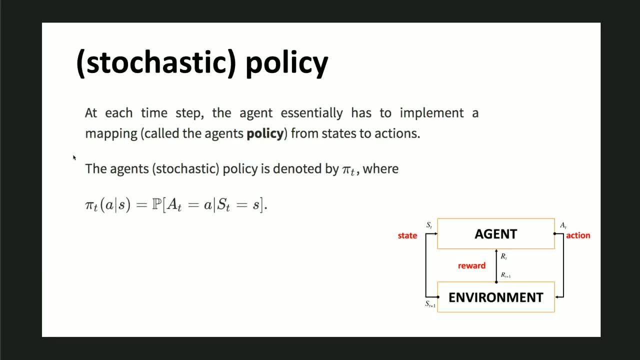 best action. you're not encouraging too much of exploration. so okay, you want to take the best action most of the time, but sometimes you also want to take other actions so that you can figure out some other possible ways of winning the game. yeah, that's why the whole notion of a stochastic policy becomes important. so that's the probabilistic. 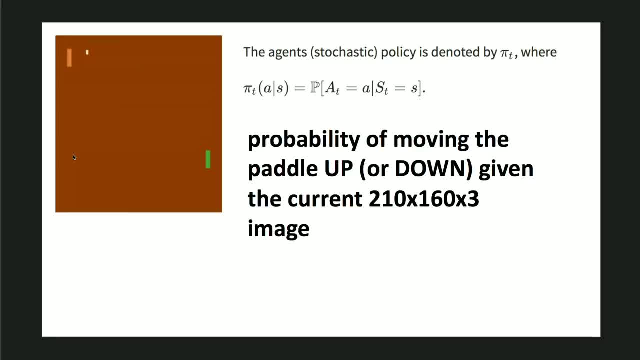 formation. okay, so in this, what is it right? so, in this game of pong, it's quite simple. it's the probability of moving the paddle up or down. right, which is probability, that the paddle is up, or the probability that y is equal to one. yeah, given the current image, which is this: two hundred ten. 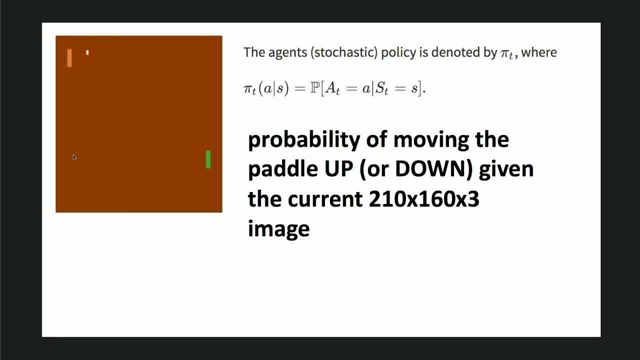 cross one, sixty, cross three image. so essentially i'm trying to learn a function from this hundred thousand numbers to a probability which says whether i should be up or down. yeah, that's all there is to what is the policy. so we figured out now what is the policy. yeah, but now comes to the 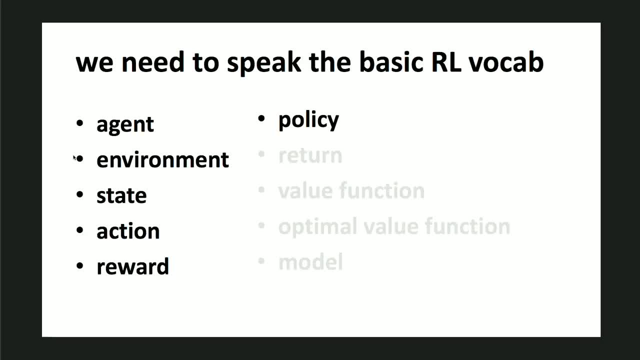 question: okay, i know what is the rl framework, i know what it means to be. what's the policy? now, how do i learn this policy? right, what? what is the formalism you can give me, or what is the mathematical machinery you can give me to learn the policy? 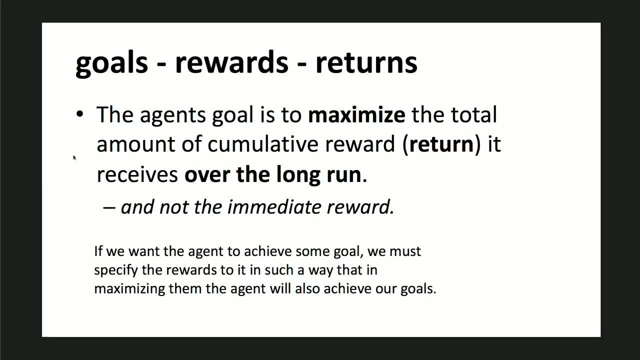 for that we need to bring the concept of a return. yeah, can you see? i can't see the time there. i just want to make sure i'm right on time now. so this is a bit frozen here. okay, so the agent's goal actually. so there are three things right: goals, rewards and returns. 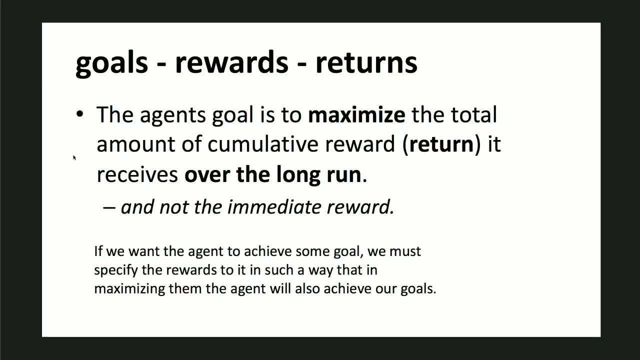 yeah, so this is what we'll walk through. yeah, so again at a high level. the agent's goal is to maximize the total amount of cumulative return reward it receives over the long run. so you saw that earlier: every time you take a action, you get a reward right. but what we don't want to do is: 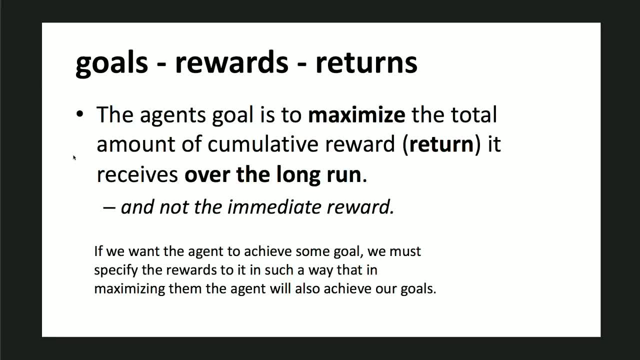 we don't want to maximize our our, we don't want to decide our policy to maximize our rewards, because they are almost instantaneous rewards. they are like, they are not long-sighted, right. what you want to do is you want to maximize the probability that eventually you're going to win, right, so that's. 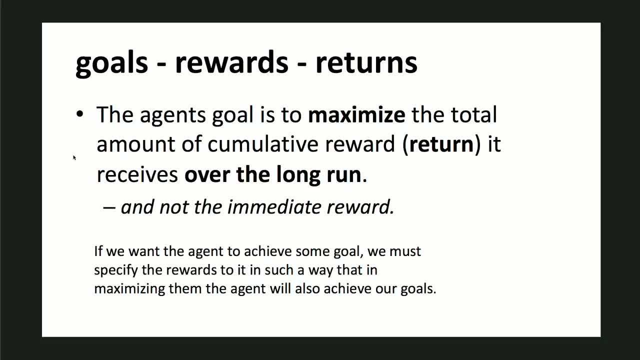 what and what we call it. we need to formalize this notion of what is actually a return. return is the amount of rewards you get over the long run, and not just the immediate reward you want. right, because you're no one is, you're just started with, you're playing one or two games you get. 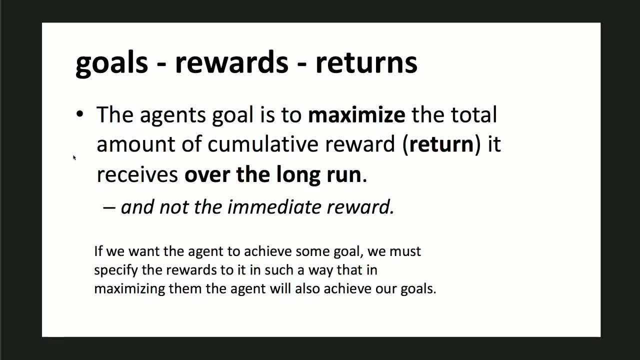 a small reward and you don't want to base on something. so- and that essentially comes to the most crucial step of modeling rl framework is actually the way to think is that you have some goal. right, that's what i say. the goal is: i want to win the game. yeah, and the only knob you have 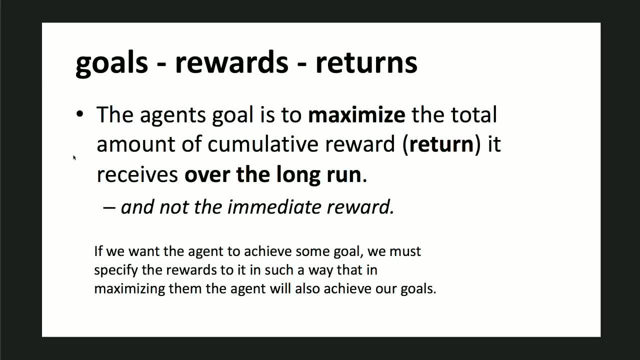 to make sure that you win the game is how you specify your rewards. the kind of the creativity comes in. how do you specify your rewards so that eventually, by maximizing this cumulative rewards, i reach my goal right? if these rewards are ill specified, or i mean if it was not specified in the right way, it will try to only maximize that there's no goal in mind. 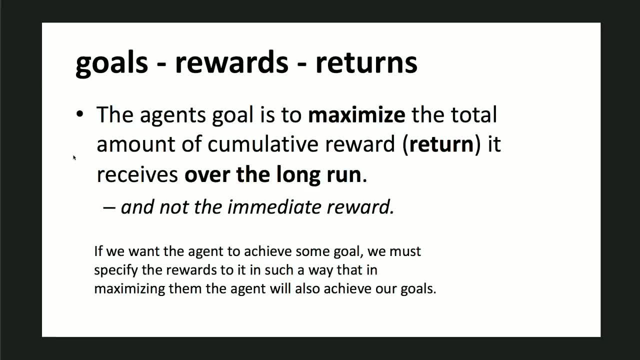 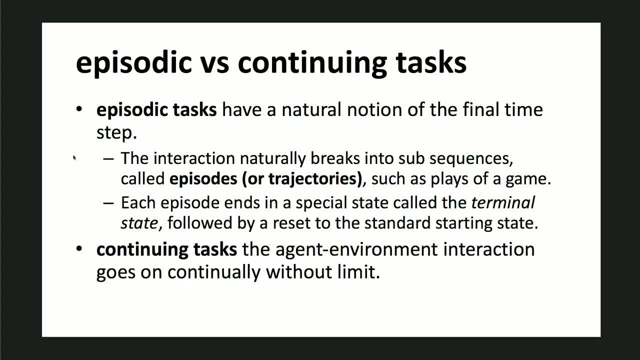 the mapping from goal to rewards is what you essentially have to play around with. how do you do so? before i continue to give them more notation, i need to kind of define two kinds of tasks people talk about. one is called the episodic tasks and the other is called as a continuing task. 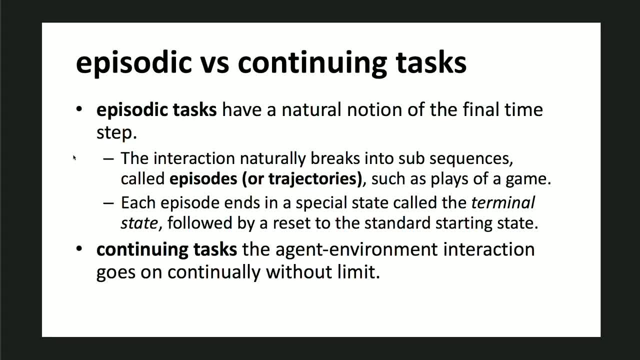 the example of pong i gave you is an episodic task. yeah, an episodic task is a natural notion of a terminal state that i start playing the game, i win or lose, and i stop, boom, i again restart, i start playing the game. so every one trajectory of a game is called an episode, and then you play multiple. 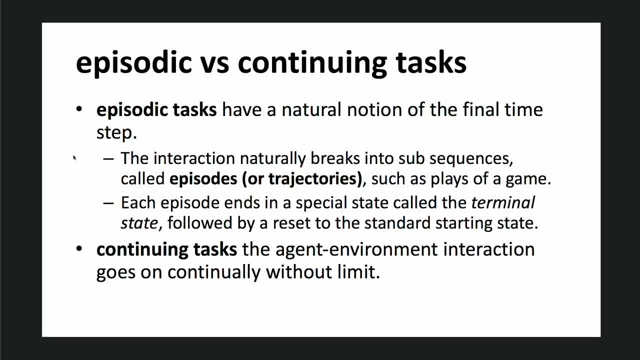 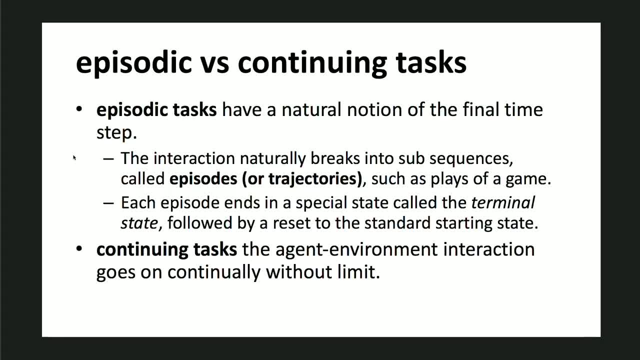 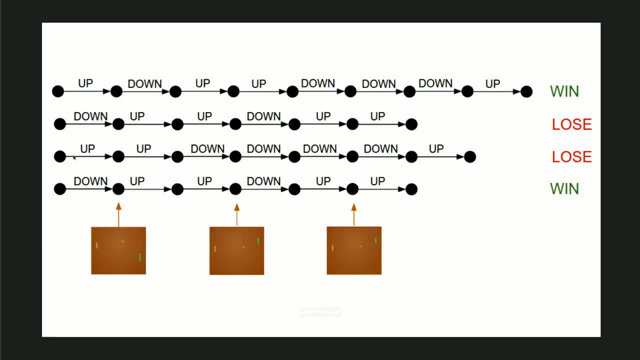 there are other tasks, but we won't talk too much about the continuing task. i think for this tutorial will be mainly focusing on an episodic task. yeah, and this is how an episodic task would be for the pong game, right? so you have, this state is just an image, right, and each time you take an action, 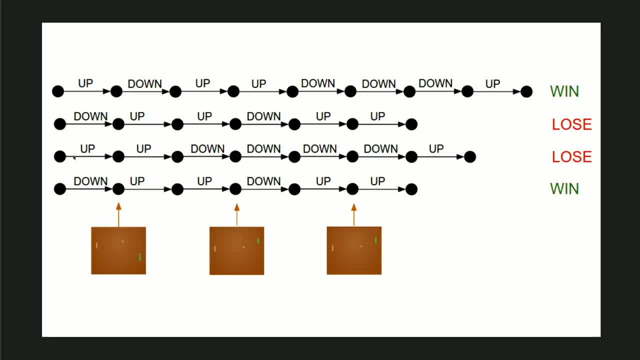 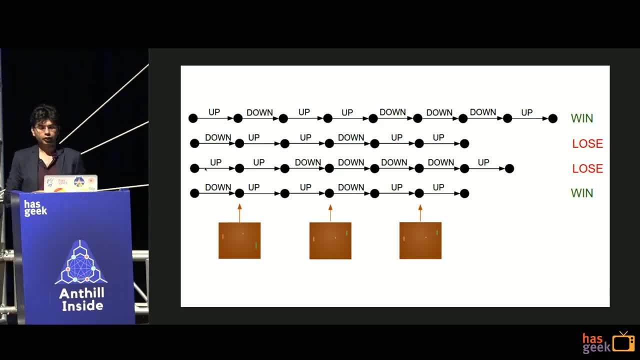 either you go up or down, up, down, down, down, down, up, up, up and eventually boom, you either win or lose. yeah, so when you win, that is one episodes. so what i shown you are four different episodes of the game. right, you start playing the game, you take some actions, you 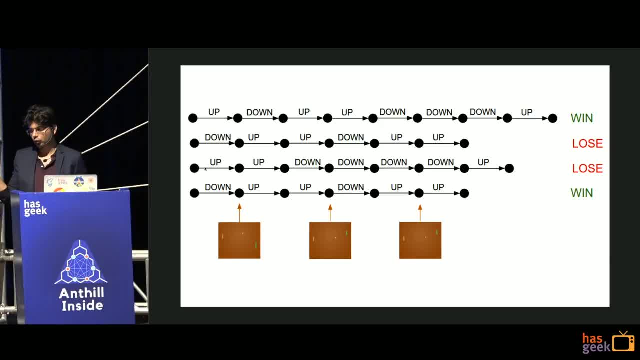 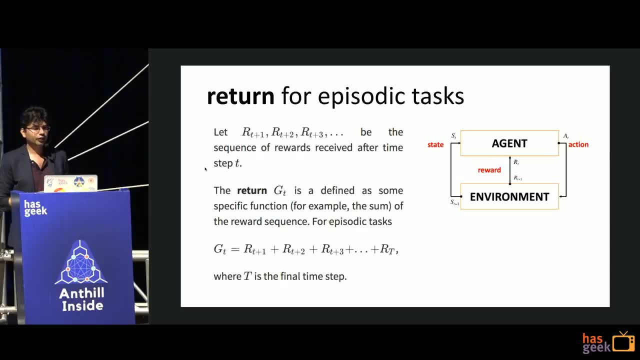 win, then again start playing the game. you take an action, then you lose, so you'll keep repeating. these are called episodes of the game. so now we'll define this notion of what is a return for an episodic task. so for that, what you have is this notion of time steps right at any time t you took. 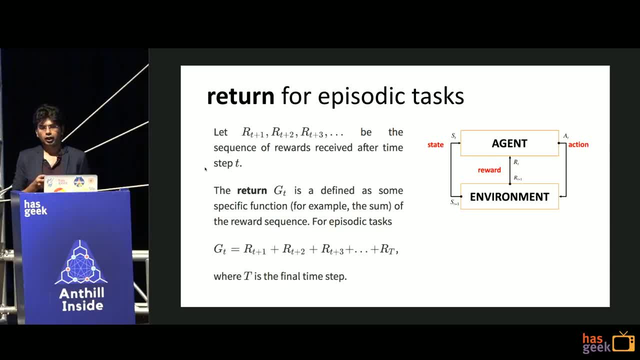 an action 80, then you got a reward- 80 plus 1, and from that you start continue playing the game, and then you got this series of rewards- t plus 1, rt plus 2, rt plus 3- till you hit the terminal state. yeah, and return is nothing but. 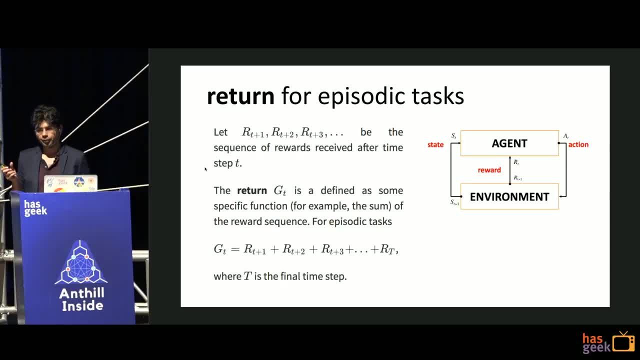 just a function of these sequence of rewards. yeah, that's it, and it can be technically, it can be any function, but the most commonly used the function is just the sum, which is essentially a sum of these rewards. right? so in our pong example it will either be one or minus one, because you start off. 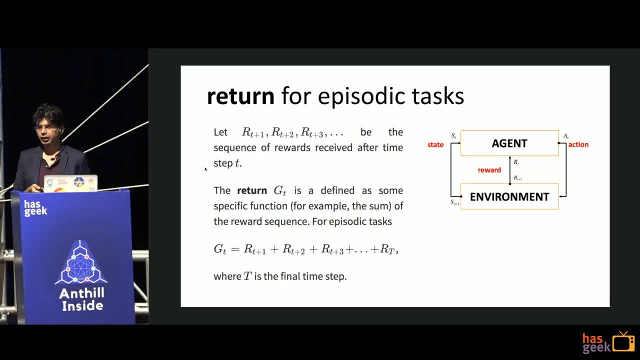 zero, zero, zero, zero, win, zero, zero, zero, minus. right, but in general a lot of applications the rewards does not have to be like zero one rewards. you can actually have the rewards and so technically a reward is just a sum of these things. so you get this reward of plus one, minus one, minus. 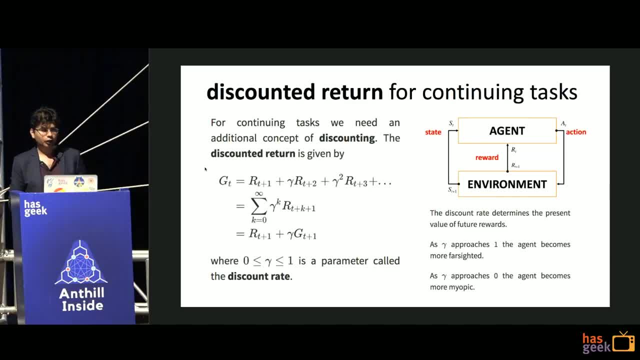 one plus one. this is fine, this is the whole sum. so for continuous task, we introduce some other notion of, called as a discounted return. yeah, which is essentially- let's say it's- very simple problem, because if you have a continuous task, if you add up all the rewards, it goes to infinity. that's not. 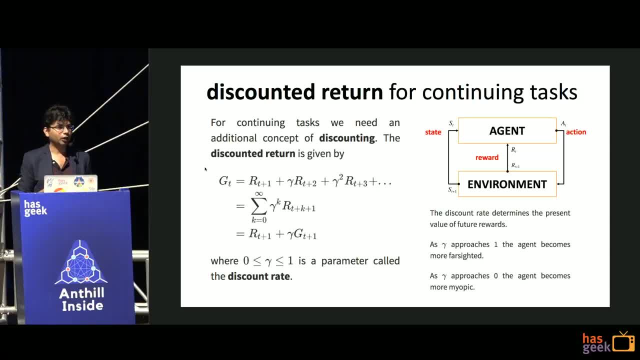 tractable, right. so introduce something called the discounting factor, called gamma, yeah, which is rt plus 1 plus gamma, rt plus 2 plus gamma, square rt plus 2,, yeah, So you can think of, gamma is some number 0 or 1 where you down weight, the future rewards, yeah, and that is. 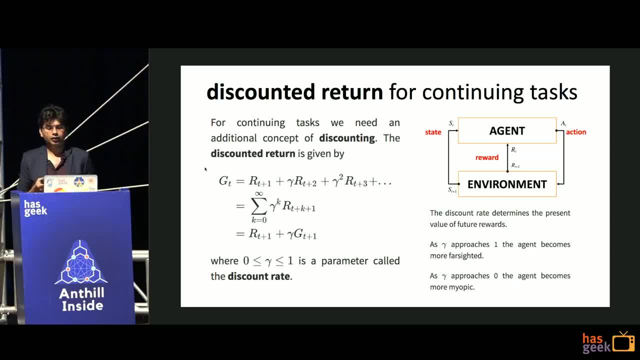 called as the discount rate. So the discount rate actually depends the way. say that it is the present value of your future rewards, right, and how much are you going to give importance to the reward which you will get in the future, as opposed to valuing your current reward? 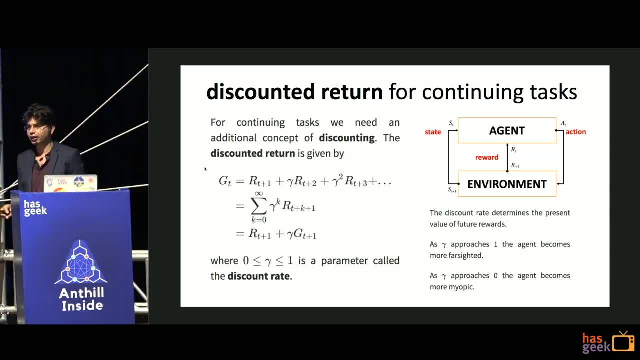 So as gamma approaches 1, the agent becomes more farsighted because it want to take this in the long run. as gamma comes to 0, it is a very myopic agent. that is a very greedy. it wants to do only maximize right now, yeah, and that has a factor of what kind of policies. 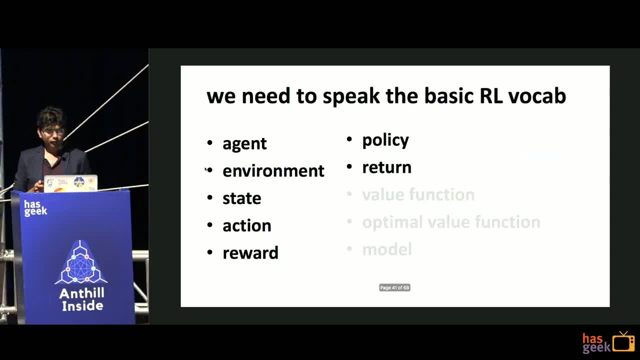 it will run right how you set the gamma. Okay, so I talked this policy now and I called it return. yeah, So policy is how do I take the action? and return is essentially what do you call a sum of the rewards you got over that one episode. yeah, that is what it. 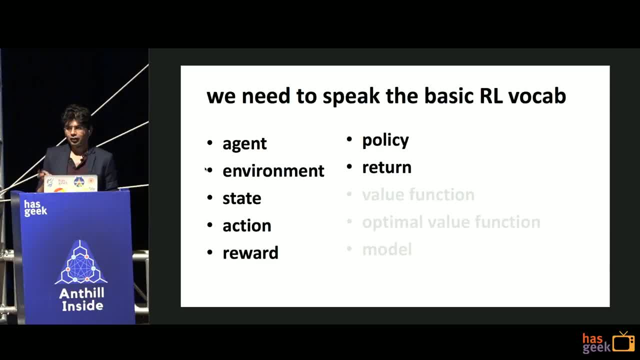 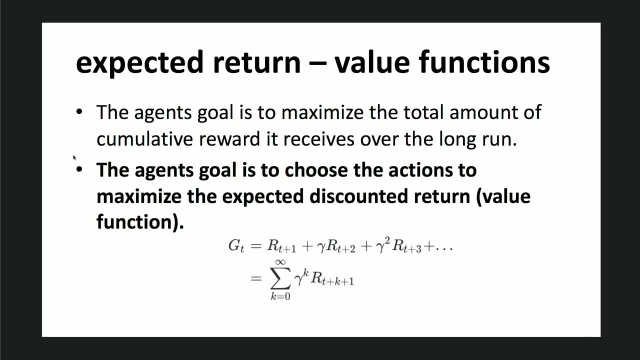 is right. Okay, so we are still not there, right, So? okay. so the reason is this: right, So what I said is the agent's goal is to maximize the total amount of cumulative reward it receives over the long run. yeah, this part of long run I did not go to right. So 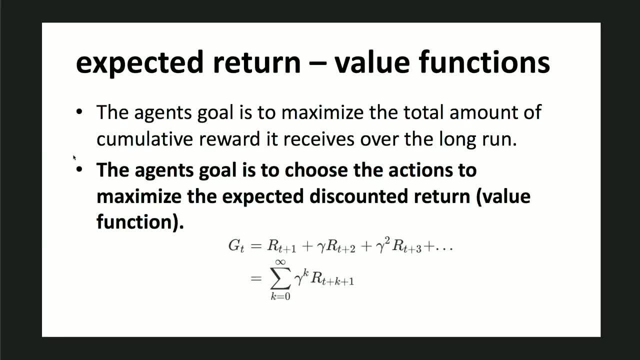 essentially you can think of. GT is again a random variable right, because the reward you are getting is for one play of the game, right. Anytime you come, you take an action, there is a stochastic policy you can branch out. then there is another stochastic policy. 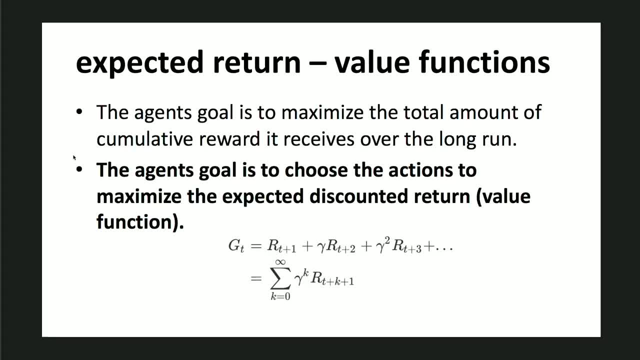 you branch out, So there will be multiple plays of the game, right? So you are going. multiple policies, right? So the agent's goal is actually to choose the actions to maximize the expected discounted return. So what we need to now do is actually take an expectation. 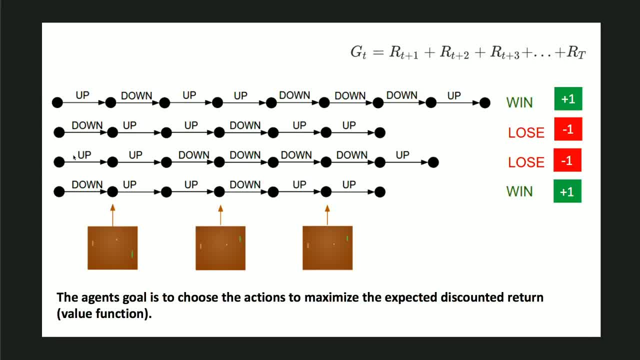 over these different episodes, right, So there is one episode you start, you win. another episode you start, lose. right, So you run this game multiple times. at each time you get a kind of a either a reward of plus 1 or minus 1, that, and then GT is just the sum of that rewards. 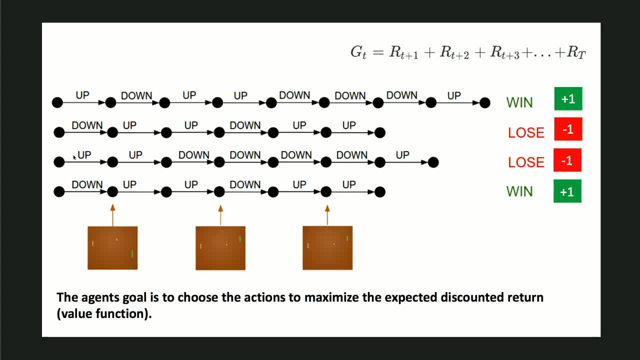 And then you can think of: just I do an empirical sum of this right. What is the average return I get? yeah, And essentially that is the RL framework is to choose the actions to maximize the expected discounted return right. So we went from reward, we went to return. then 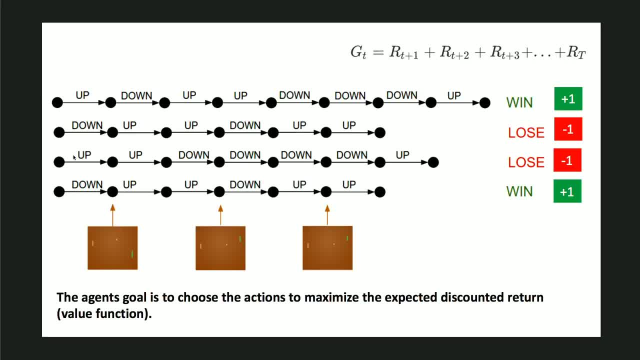 you said discounted return, then you said expected discount return, and that is what you want to maximize. And this expected discounted return is what is called in the literature as a value function, and that is what you are trying to maximize And this is the most formal. 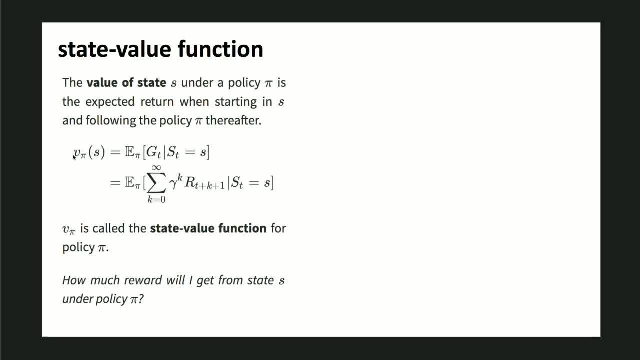 definition of reward, What we call as a state value function. yeah, which is the value of a state S under a stochastic policy. pi is the expected return when starting in state S and then Paul continuing that policy thereafter. yeah, So you started state S and then you play the game. I want to know what. 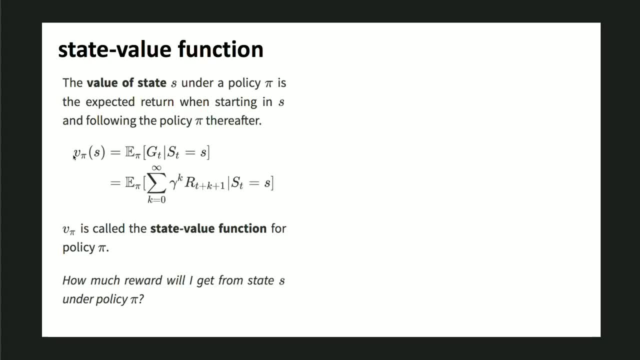 is the value of that. That is the technical term for value, which is nothing. but you start that you keep track of all the rewards you are get but realize that this rewards is stochastic. so you take an expectation of that. yeah, And that is essentially the state value function. 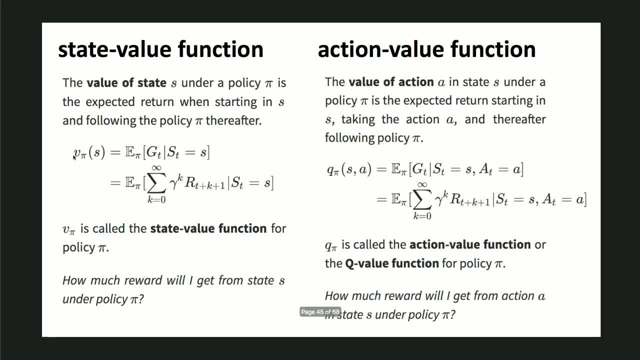 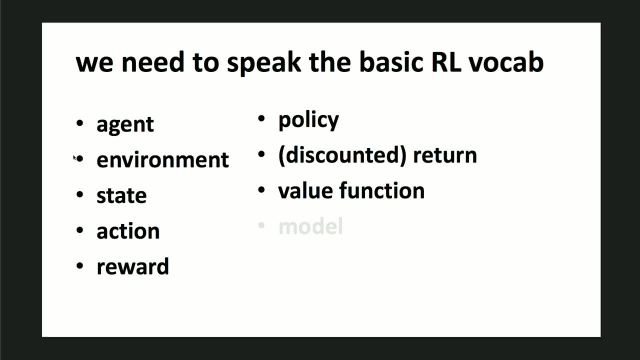 which is: how much reward will I get from state S? So I want to know what is the value of that I get from state S. under policy pi, There is something called as an action value function, which I will skip. yeah, This also I will skip. yeah, So for now, this is all we need to know. 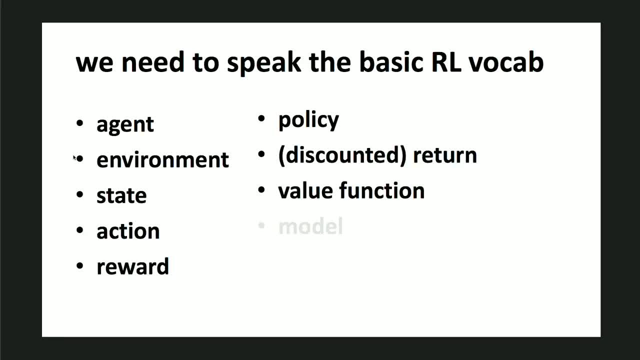 because I am kind of running out of time, So you have this policy. then I said: what is the return? which is the discounted return? then I said: expected discounted return is the value function and an RL agent will try to maximize that. yeah, So I will also skip. 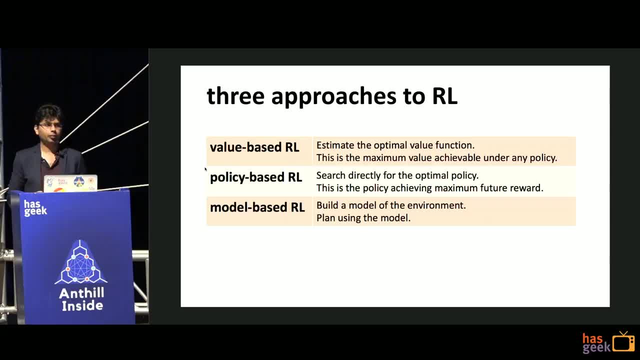 this part, okay, because we do not really need, because I need to come to the deep end. So there are, broadly, there are three classes approaches to real framing, which is called as a value based reinforcement learning, policy based reinforcement learning and the model based RL. yeah, So now I told you what is the value function. So the value based approaches. 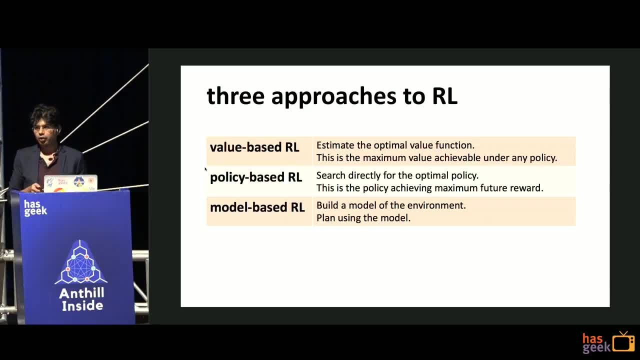 start trying to make learn this value function. yeah, Policy based RL actually takes a different paradigm. they directly try to estimate the policy without considering the value function and model based try to build a model of the environment. I think for now, let us focus only on the policy based reinforcement learning. So let us see what is the value function. 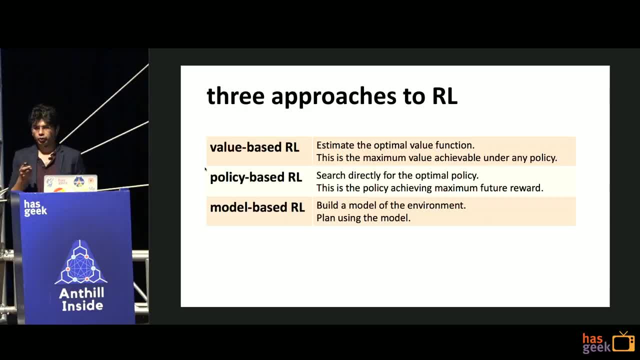 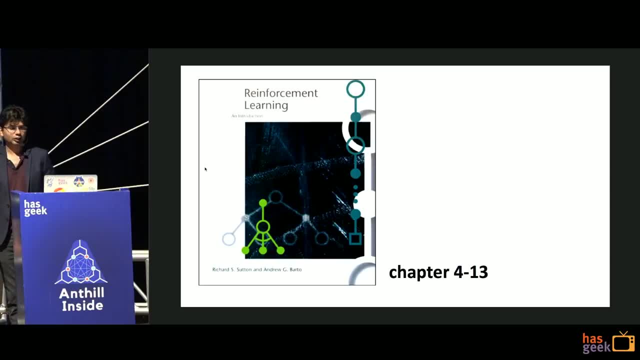 So what is the value function? So here is the value function of a data structure, and the value function of a data structure is the value function of a policy based RL and that is actually That is the one which is showing a lot of success and that is probably little. 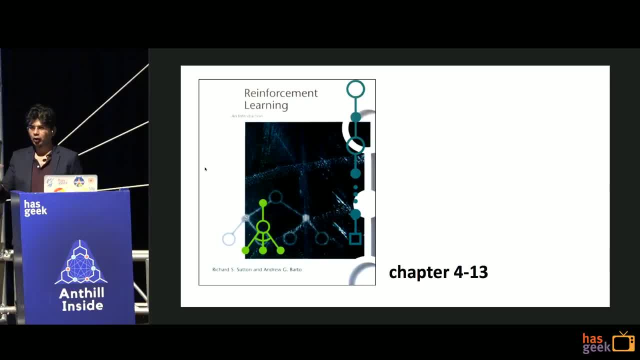 bit more hot And I covered till now essentially chapter 3 of this book. right now we can go ahead and say all chapters 4 to 13 is what is called as a classical reinforcement. learn to read all this chapter 4 to 13. that will show you all these classical ways of solving. 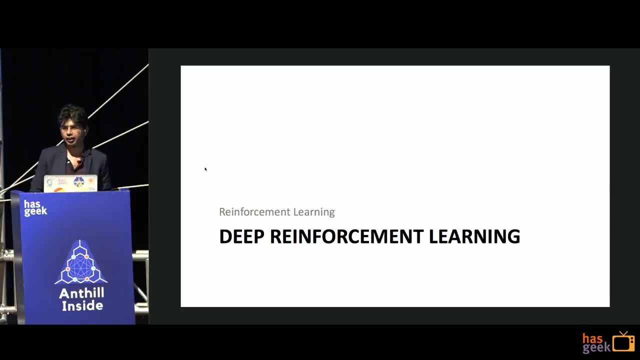 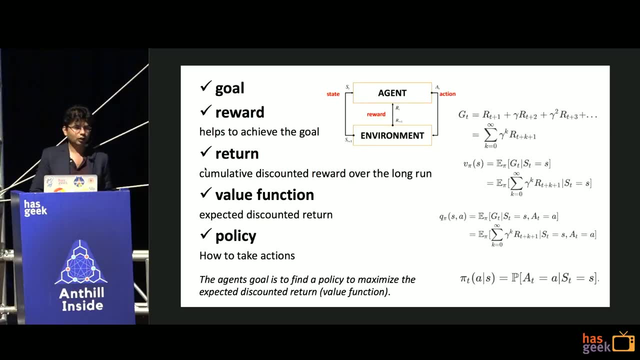 the reinforcement learning problems. yeah, now we are just going to jump directly into deep reinforcement learning with this motivation. i think it's pretty simple to see what's happening here, yeah, so again, i'll recall a little bit of notation, right? so so for me it's always this: 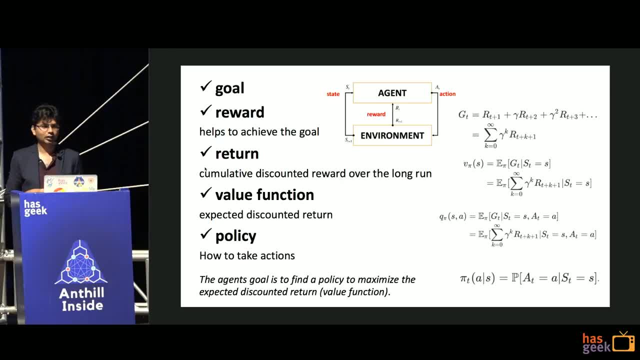 notation. i think that's why i keep putting this again and again. it's always have to be very clear about what are we talking about. so that's a goal, that's a reward, which is the rt return is the cumulative discounted return over the long run value function is the expected discount return. 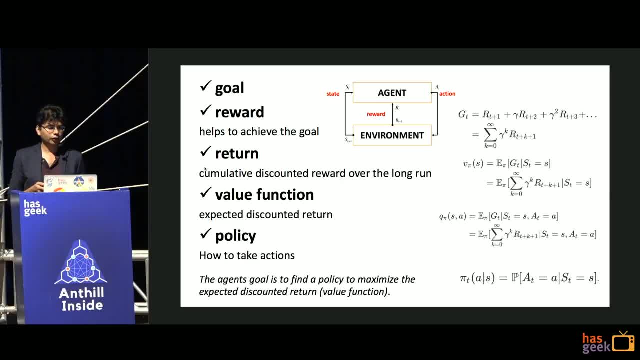 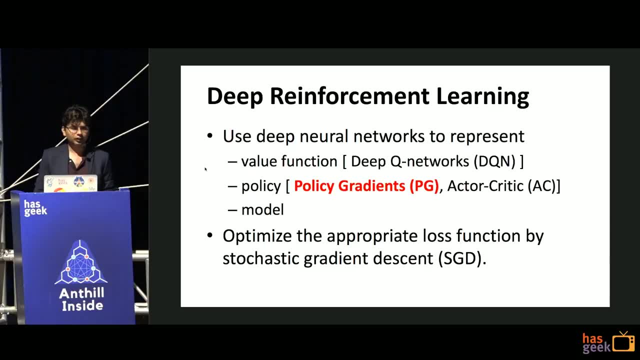 policy showed you how to take actions and the agent's goal is to find a policy to maximize the expected discounted return. yeah, so deep reinforcement learning, essentially, is that right? i told you there are three ways of doing it: value based rl, policy based rl and model based rl. so why? 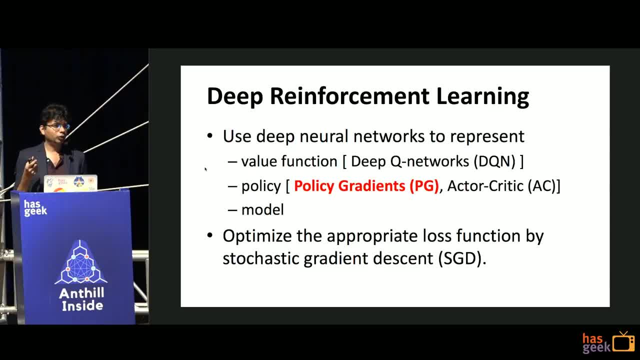 not use deep neural networks for to approximate the value function. use a deep neural network to approximate the policy function or use a deep neural network to model the environment. yeah, and those essentially are the different thing, right? so the earlier successes that the atari paper came from something called as the approximating the value function, that's. 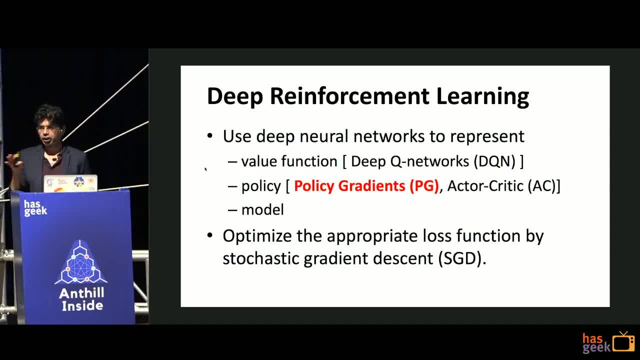 technically called a deep q network or the dqns. yeah, i'm going to skip dqns for the for this entire tutorial, and we're going to focus on something called as a pg, which is the policy gradients. we directly try to optimize the policy. yeah, and there is another algorithm called actor. 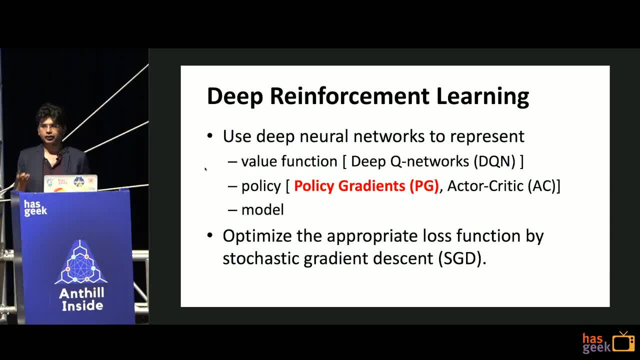 credit. yeah, so if you want to go back and learn again, i think pg and ac are the things you really want to focus on here, because that's essentially where they are the much easier to optimize the data and that's where they're showing a lot of potential. yeah, so we'll focus on this algorithm. 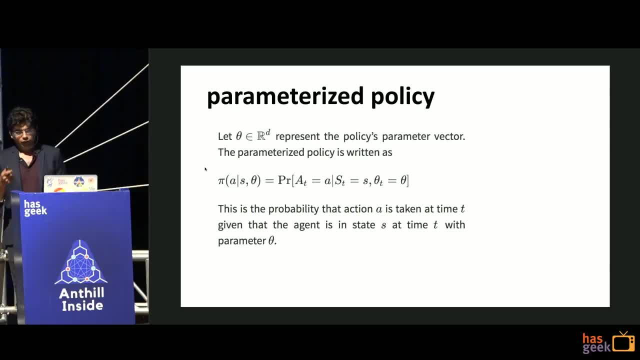 called policy gradients. yeah, so what i said, yeah, so first notion we need to get is that i defined this policy stochastic policy, which said: how do i take an action? so now i need to start to parameterize this. yeah, so i'm going to say that this policy depends on some parameters: theta, yeah. 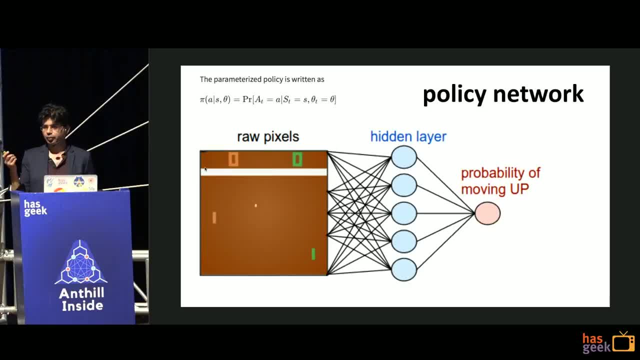 and how does it works in our place? form? pretty simple, right. you take your image, you in simple scale. you could just pass it through another neural network or a deep neural network or it could even be a cnn, right? so i took this kind of 210 cross. 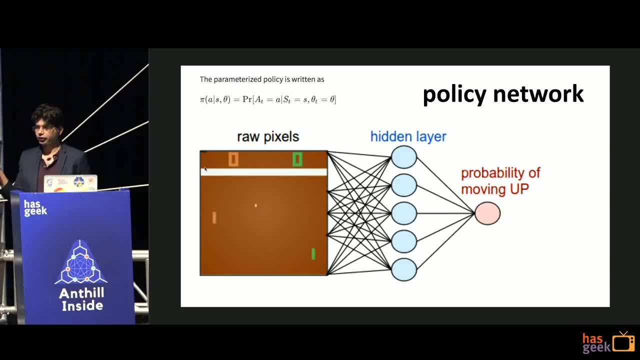 100 cross 3 image, pass it through a deep neural network- it could be a cnn or any neural network- and the output i put a soft max layer which is either one or zero. one means i move the paddle up, zero means i move the paddle down. that gives me a parameterized policy of moving my paddle either. 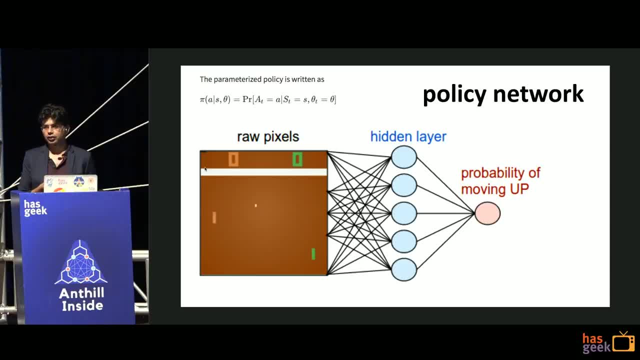 up or down. so what is this modeling? given any image st, what is the probability that i take the value of that? this is essentially the policy network. yeah, and the whole goal is now try to learn the parameters of this policy network in the reinforcement learning paradigm we discussed earlier. 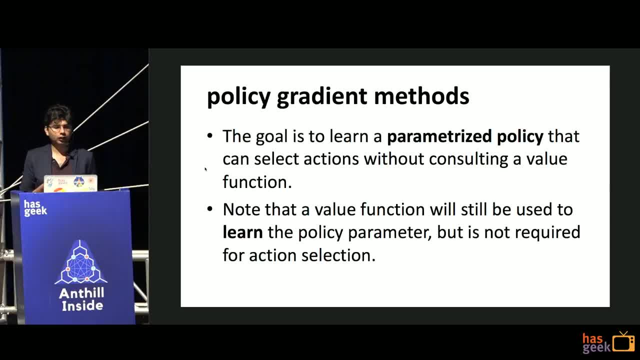 so the goal is to learn a parameterized policy that can select actions without consulting the value function. yeah, but technically not that a value function will still be used to learn the policy parameter but is not required for action selection as in the q based other value based. 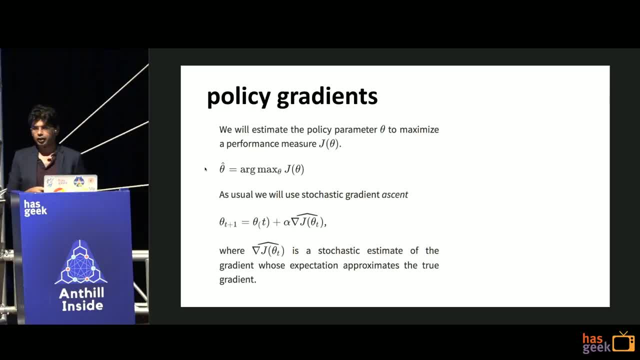 algorithms. yeah, those are familiar with that. So I have a policy parameter, theta, which are the parameters of this CNN, yeah, and I want to maximize the performance measure called J of theta. As usual, we will do stochastic gradient descent. the only thing is this is what you are trying to maximize it. So I 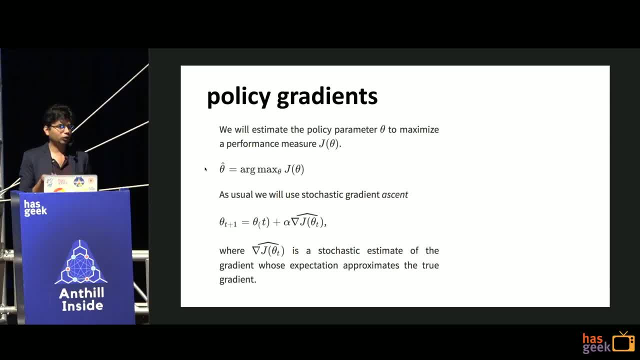 will do a stochastic gradient ascent. So theta t plus 1 is equal to theta t plus alpha into gradient of this thing. yeah, So essentially the whole literature, probably I can. you can write 20,, 20,, 30 pages, and how do you? what are the different ways of computing this gradient? 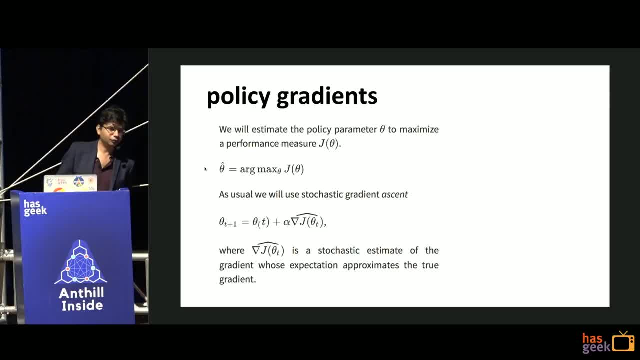 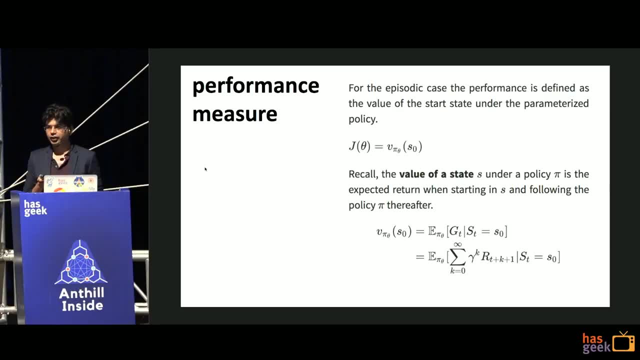 that is all the policy gradient is about. yeah, fine, yeah, So I think so. I think so again. now we will come back to the same right. So essentially we said we want to maximize the discounted return, So we are going to the performance measure. would be that value function. 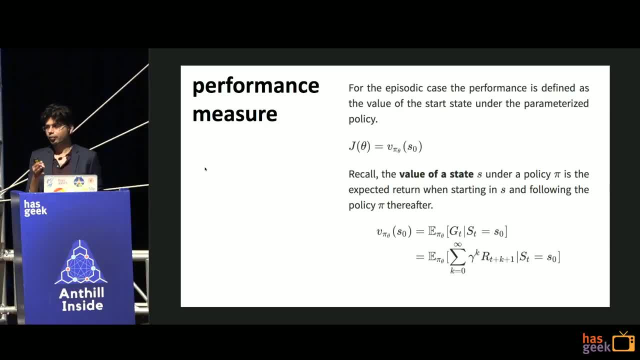 we are trying to maximize. So, given a start t, I am going to play the game and I am going to get a lot of rewards. how do you want to maximize? yeah, So the whole thing is, how do I find the derivative of the value function? So I am going to find the derivative of the. 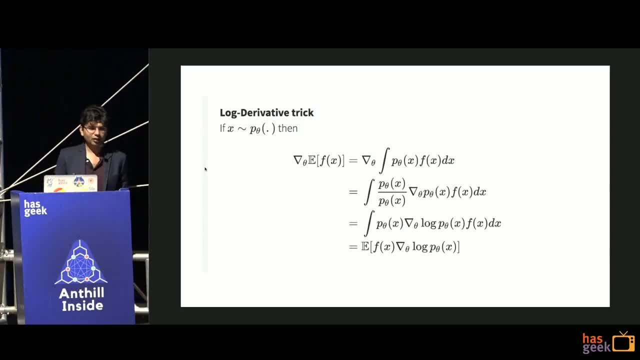 value function. So I am going to find the derivative of the value function, So I am going to calculate the derivatives of that right, and this is a little bit, not because lack of time will give. this is probably is the most crucial model. how do you compute the derivative? 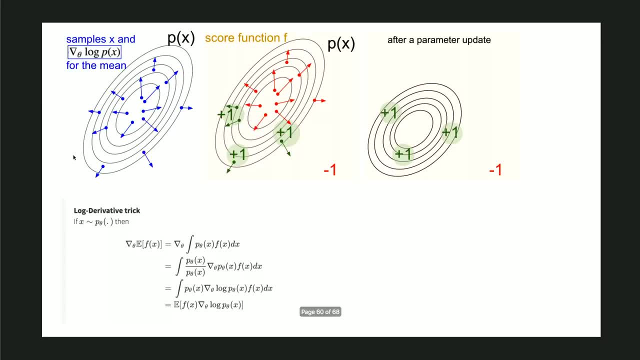 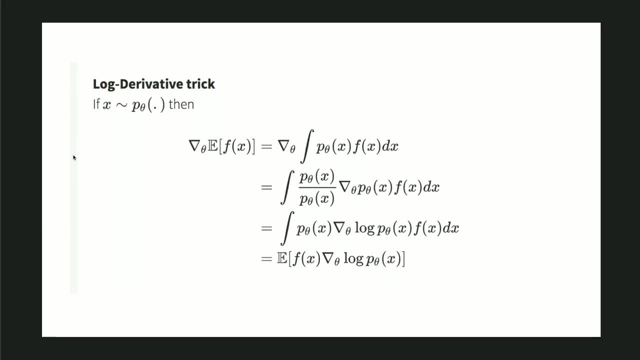 There are two standard tricks people use. yeah, The one is called as the log derivative trick and the other is called as the gradient of the episode. yeah, So the log derivative trick actually have takes the gradient of an expected value of a function of f of x. yeah, So so. 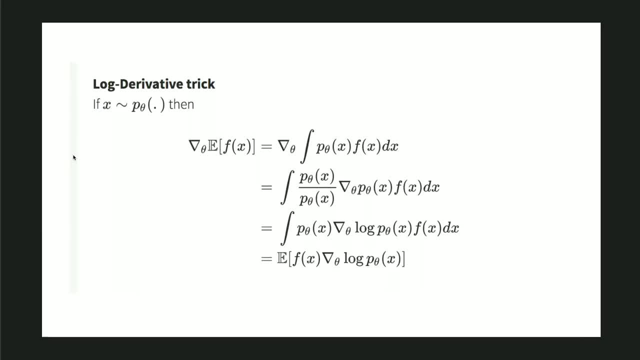 this is: gradient of expectation of f of x is nothing but expectation of f of x plus this term. yeah, This is the trick we will need to do right. We will forget the derivation, but eventually this gives you a way to push the gradient inside the expectation. yeah, 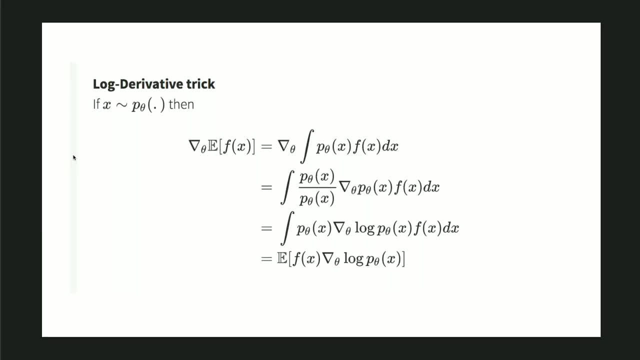 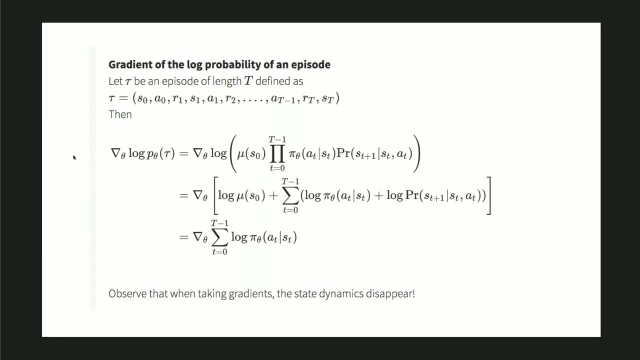 And that is very helpful because it helps us to do now the expectation via empirical averages. The second is, actually we also need to compute the log probability of an episode. The way to think about is that I run the game, I get a bunch of states, So I just want to see what. 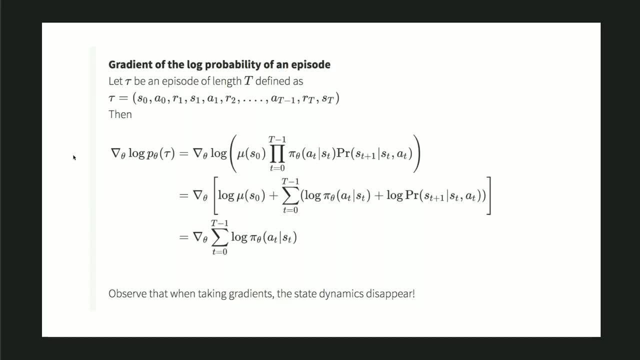 is the likelihood of this trajectory right. So, and that is where all the dynamics of the way you are defined coming right. So, essentially here you say that what is the probability of the first state, and then, given this state, I take an action. a, t, this is my probability. 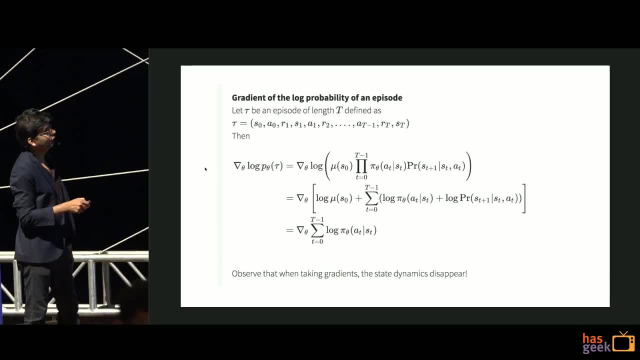 that is the policy. And then I take this action: a, t, I am in state t. what is the probability that I move to is t plus 1.. And this again I am invoking the MDP, the Markov property, because it does not depend on anything else. So this is all the trajectory, and then I essentially 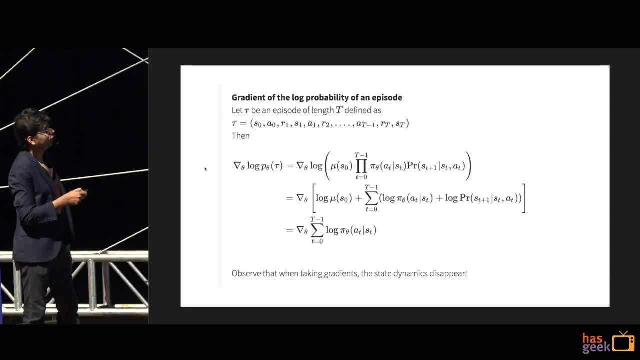 bring the log in and sum it up and take the derivative, And all this it comes up to is that the derivative depends only on the policy. That is probably the beauty of this. Essentially, the state dynamics completely disappear Once with policy gradient. I really do not need to know what is the Markov property, what, how the states. 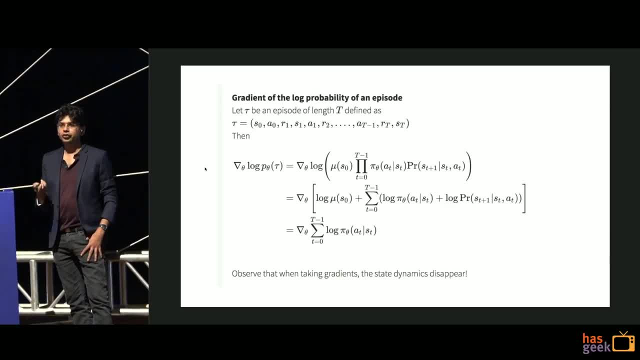 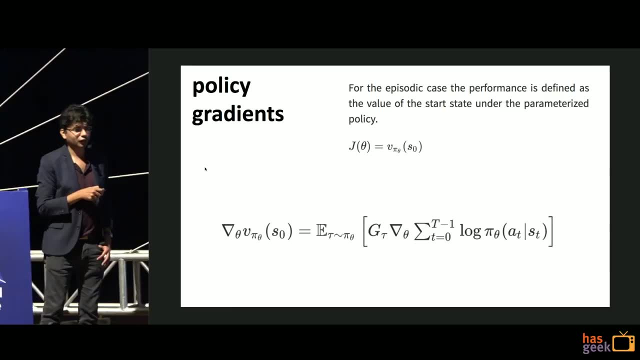 revolving etcetera. All I need is the gradient of my policy network. yeah, And probably that is the whole thing. This is essentially the final takeaway of this whole talk. is this equation, if you remember right, Which is essentially the gradient of my value function? 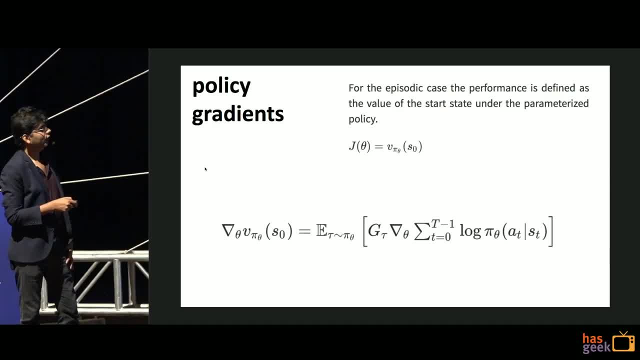 with respect to the parameters theta of the policy. So this is essentially the final takeaway of this whole talk. is this equation, if you remember right, Which is essentially the gradient of my function with respect to the parameters theta of the policy, And this is essentially the point at which I actually take the gradient of the here I 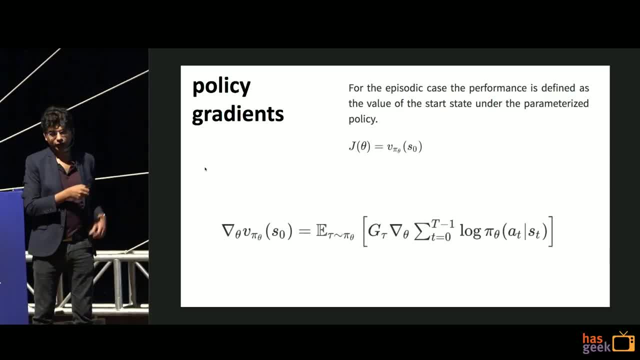 have a cheap chart on this, And this for fear of shortness of speings. there is a system called the approximation of a rosin graph. now let us discover this: a rosin graph is actually going to have a ANY ultimate, Yeah. 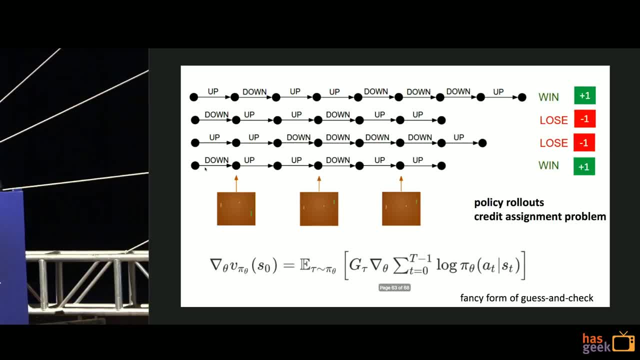 So the interpretation of this equation, I think you can see it in this one here. So this again comes to a standard. So if I think about in a standard supervised learning setup, right, I can think of that. I have a CNN and I am predicting 1 or 0. should I go up or down, right? 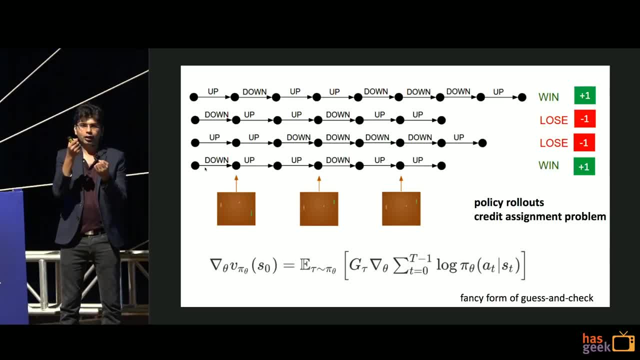 I can actually give you a lot of examples. I give you this image: I say: move the paddle up. I move the paddle down, up down. So that would be a standard, supervised way of learning this network here. But the thing what has happening here is that you really don't get. 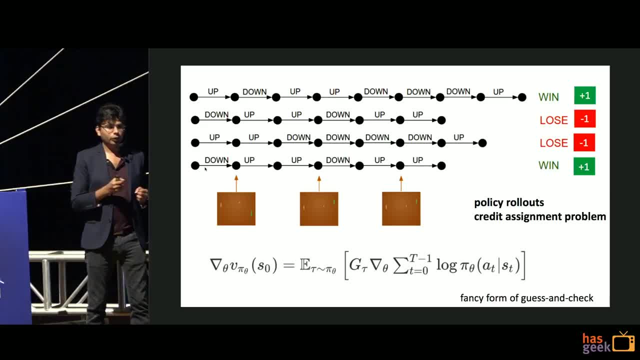 supervision at that instance level. All that you get is you play the game to the end, Then you get a reward of either plus 1 or minus 1.. Now I need to figure out how do I have to propagate that reward back to every action I take, Because right what you are getting. 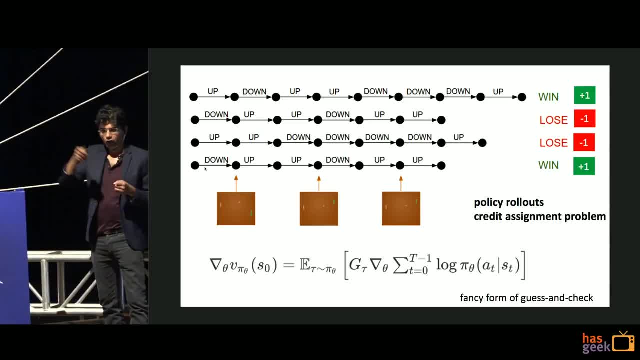 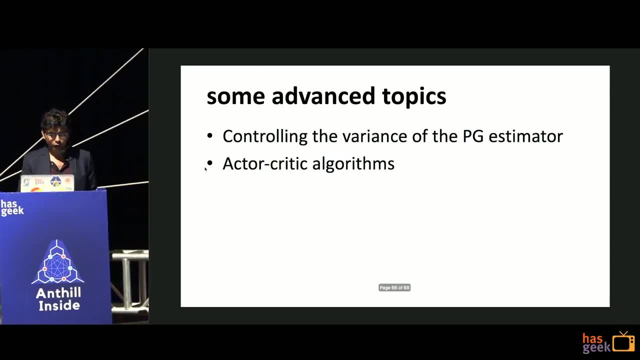 is you, for example? you figuring out, there is a long run and then this: yeah, Right, ok, let me just end with one slide. I have two more slides, I will just end it. yeah, So the reason why policy gradient is important is that maybe 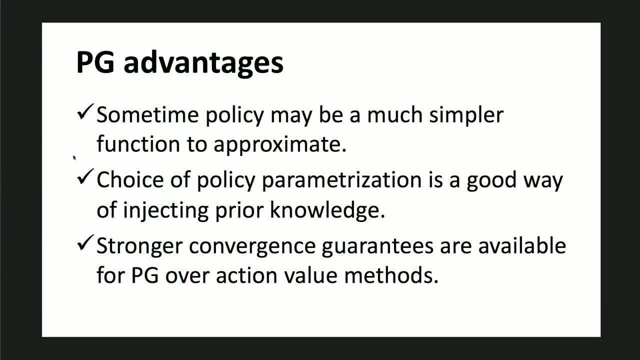 I think we want to learn one method in deep reinforcement learning. that would be the policy gradient right. We want to read up more And essentially it is actually much simpler to approximate the policy gradient, And the choice of policy parameterization is a good way of. 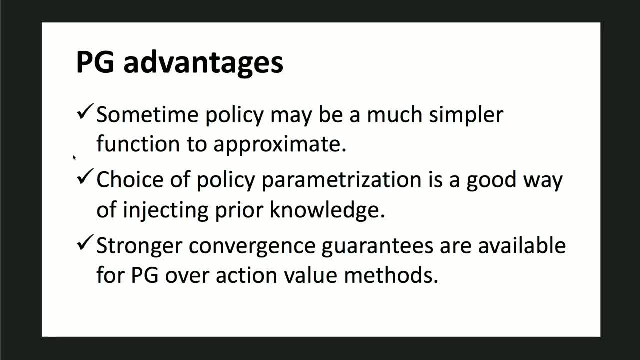 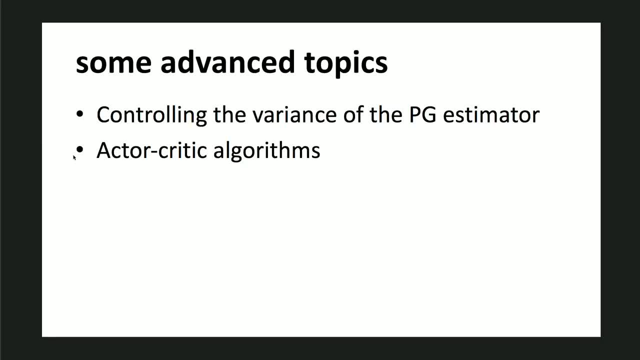 injecting the prior knowledge. There are very stronger convergence guarantees are available for policy gradient over action value patterns. So the next step from more advanced topics, if you move next from here, is the equation I showed. you actually does not work that well in practice. The theory is the same, But you 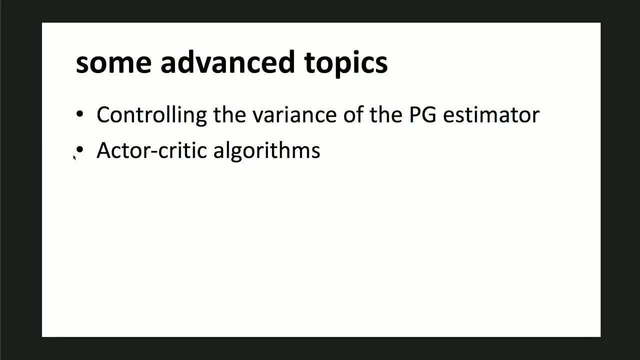 have to control the variance of that. So use something called as the baseline estimator to subtract, to decrease the variance. and that is what you will find, probably papers written on how do I control the variance of the gradient of the value function. That is essentially all the literature is about to get better. 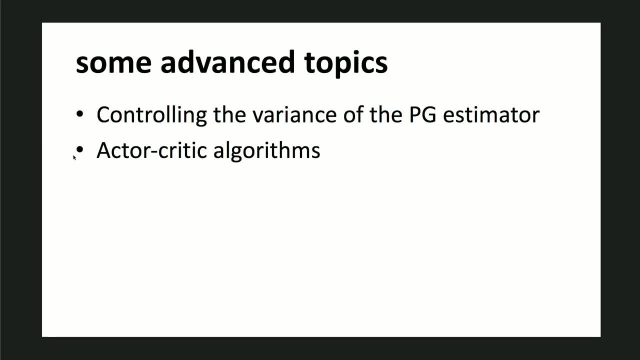 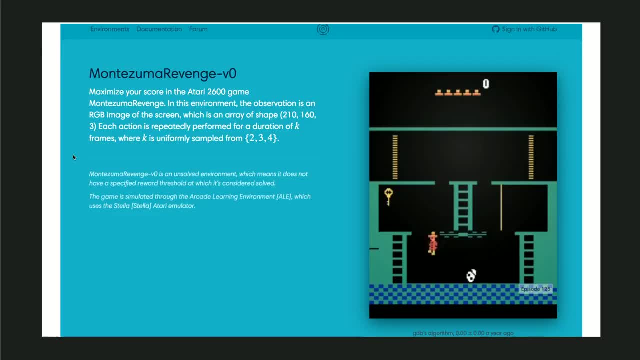 estimators of the gradient of that value function. And then there is a next line called active critical algorithm, which use both the value function and the policy gradient, which is not comfortable. I will end up with two slides, right? So can reinforcement learning solve all kind of problems, you know right, And that is what I want to go and think about What. 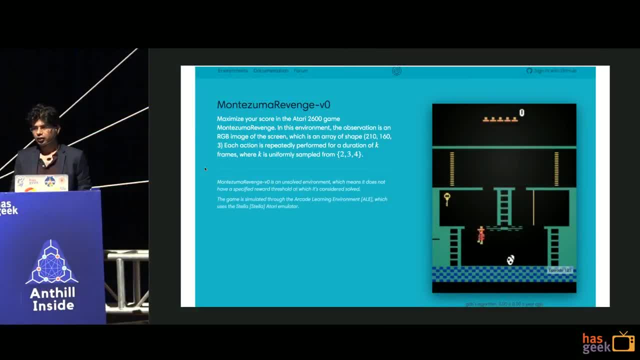 are the other kinds of setup you think probably RL cannot solve right. So this is the one game, which is called as the Montezuma Revenge, where it is known to fail very miserably. Here, if you just summarize, everything is fine, but what is happening is that the key part of 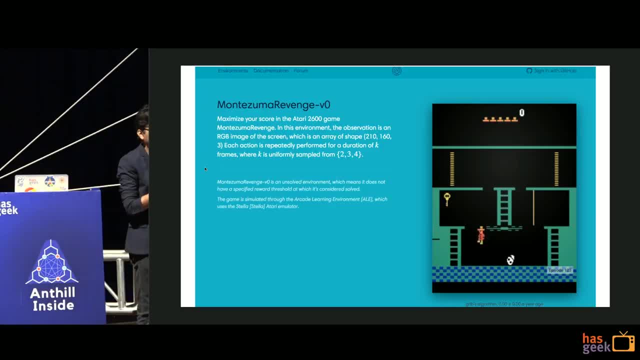 the game is that the agent has to figure out that there is some key here. The key will unlock me to some hidden treasures and I open that, I get some reward. And humans we, when we are playing the game, it is very natural for us that key means something right? So we really do not explore. 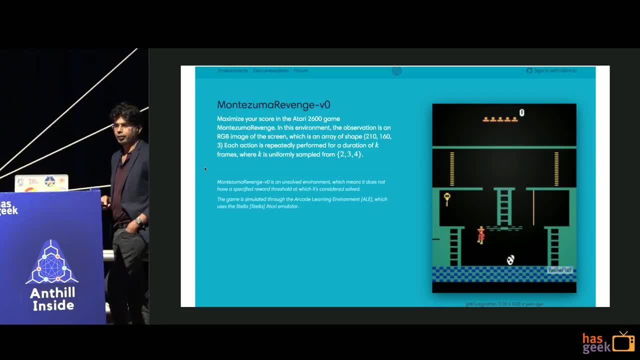 too much. We just directly go to the key. But in order to for a machine to figure out or an RL agent to figure out, it has to run lots of trials till it figures out that hitting the key is the right thing. And that is why this lot of in this game. I think it is very easy, not I mean? 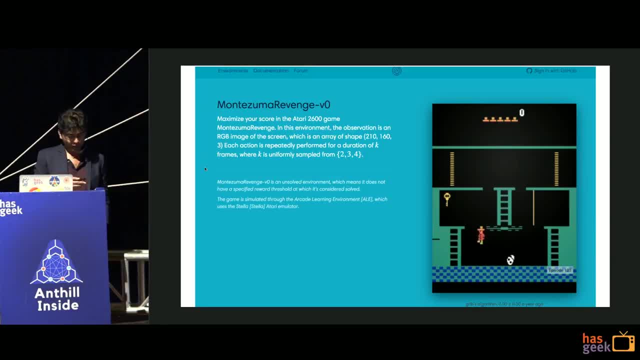 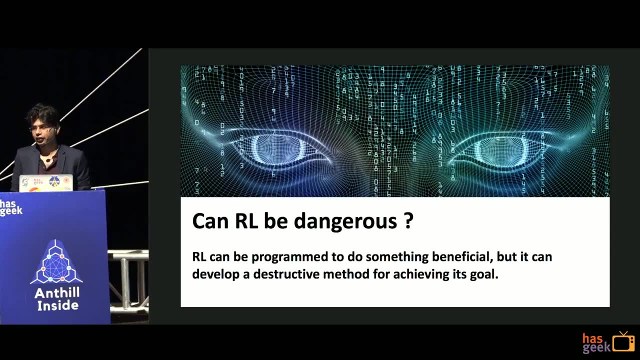 humans can do better than RL in this case. yeah, And I think I will just end with this slide as a thought for you. right, You want to think about, with all the hype and all these, can AI be dangerous? right With, probably with supervised learning, people think it is ridiculous to think of.